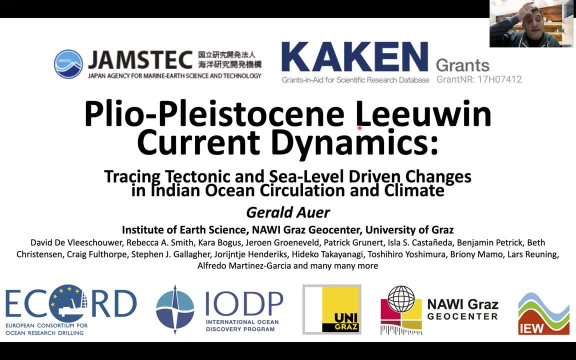 circulation patterns and how these changes may have affected the Earth's past climatic evolution. In his research, he focuses mainly on tropical to subtropical shallow marine carbonates. Following his participation in the International Ocean Discovery Project, Expedition 356 in 2015,, he became heavily involved in research dealing with the Neogene evolution of the Indian. 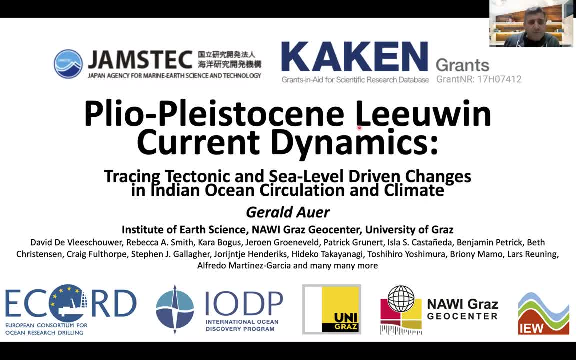 Ocean and the influence of climate and tectonic influences on large-scale cross-hemispheric circulation patterns, such as the Indian or Australian monsoons, and the evolution of the Sha'ul Indian Ocean. Bjerkenes Mechanism. Okay, if I did a mistake, please correct me. 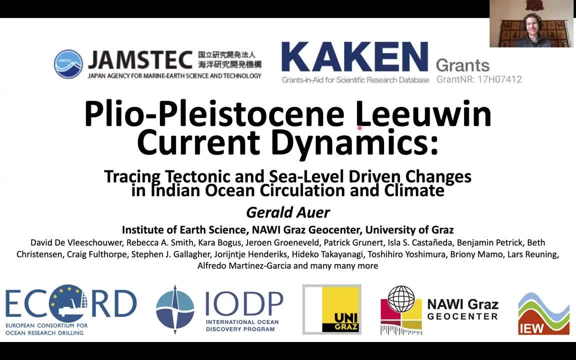 That's totally fine. Thank you very much for the very nice introduction And again, thank you very much for inviting me. I really appreciate this opportunity to talk a bit about my research and, without further ado, I would like to present a bit of my research that came out of my stay at the JAMSTEC in Japan. 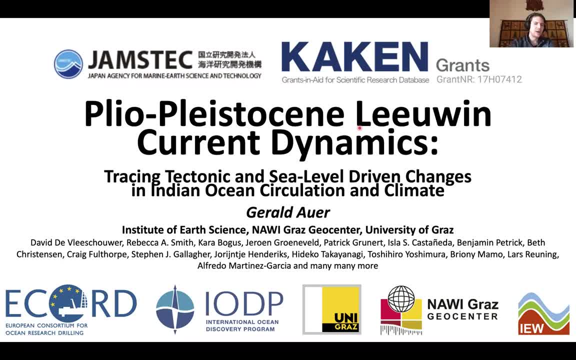 about the pleioplastocene-lubin current dynamics and how this all interacts with tectonic sea level driven changes and also the Indian Ocean circulation and climate. And, as you can see, here I have a lot of co-authors and they were all really, really incredibly helpful. 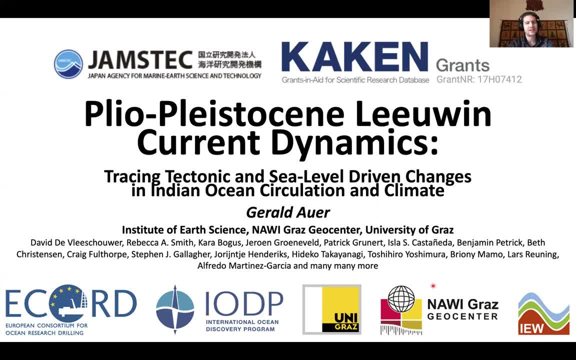 in generating this data and interpreting this data, And IODP is, of course, a very collaborative endeavor, And I think the collaborations that arose from this very nicely highlight the opportunities of IODP and also ICDP in certain cases, And so I want to like to honor this a bit. 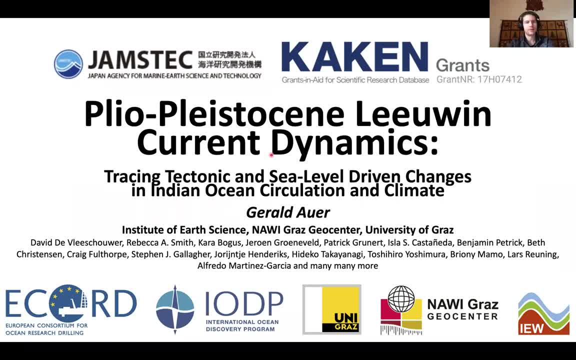 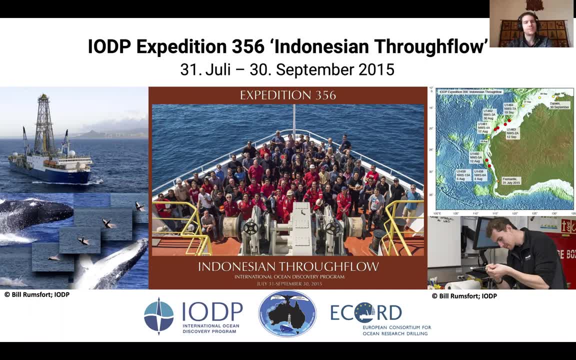 with this talk. Okay, that's mine, Very nice. So, as mentioned, a lot of this research came about from IODP Expedition 356, Indonesian through flow, which we drilled into the in the austral winter from July to September 2015.. And we drilled a transect along the west. 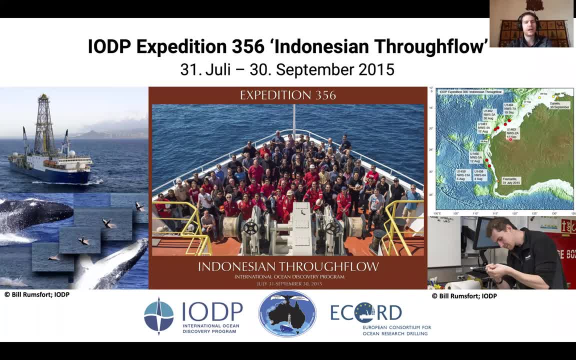 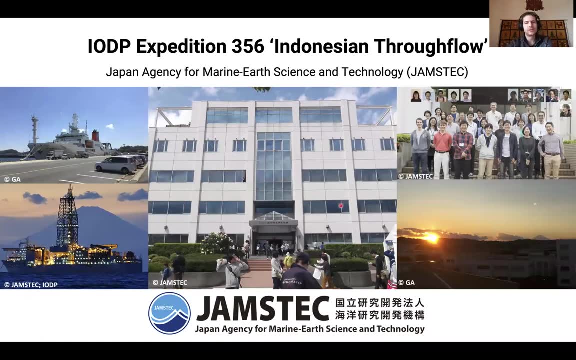 coast of Australia, along the northwest shelf and the Karnawan ramp, where we drilled several sites And yeah, it was quite a lot of fun. And now I'm going to talk a bit about the data, about this. So, again as a reminder, most of the research came about from my stay at JAMSTEC here, So these 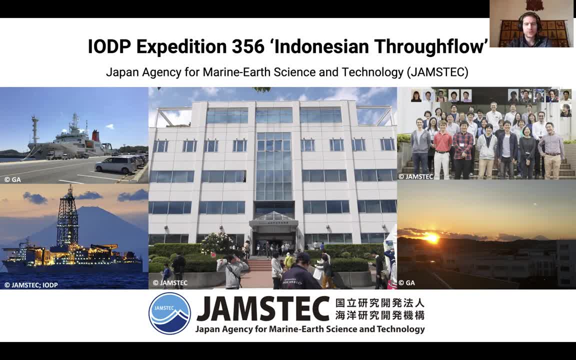 were my colleagues back then. this is the Institute, And the very nice thing about JAMSTEC is it has a very large research fleet and has a heavy involvement, of course, in IODP, especially with the GQ, And so this was a very nice place to stay and do research. 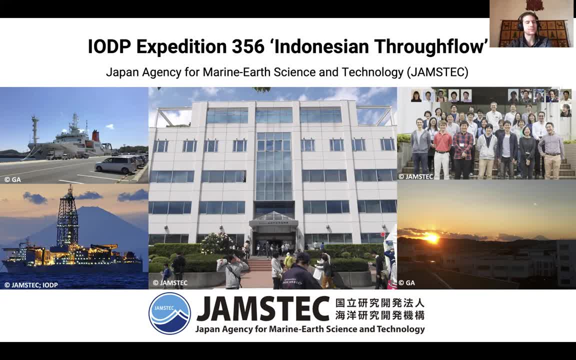 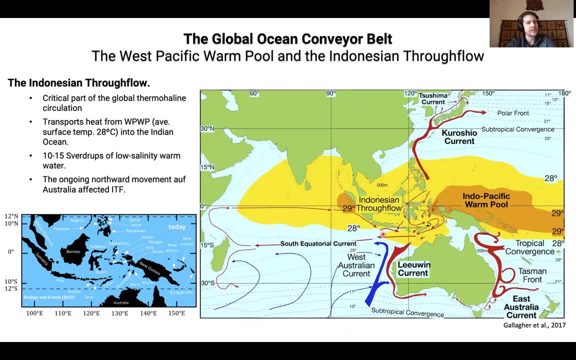 on these IODP samples during that time, Maybe as a bit of an introduction. why we drilled during Expedition 356 was our interest in the Indonesian through flow, as it is a very important part of the global thermohaline circulation. It is basically the warm water transport in the 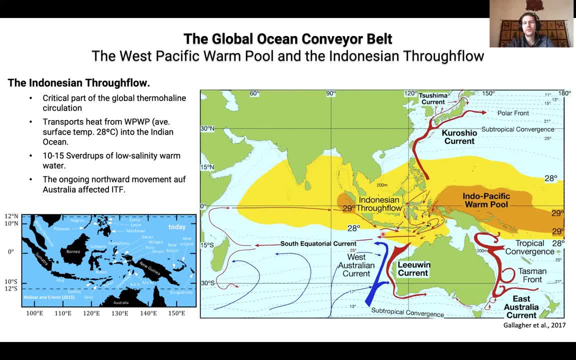 tropical area from the Pacific, specifically the Indo-Pacific warm pool, into the Indian Ocean. So it's basically the warm water loop that completes the global thermohaline circulation and transports all the warm water back into the Atlantic and further in the Gulf Stream. 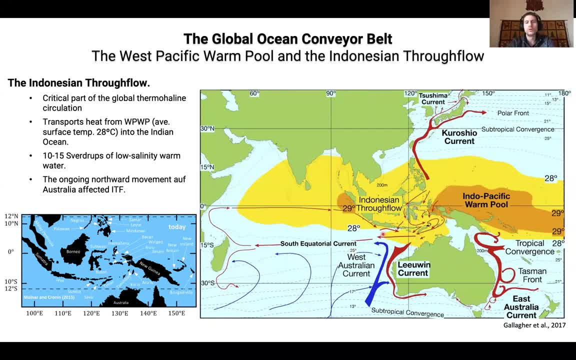 So it's a very important switchboard that controls climate and also latitudinal transport through the Indian Ocean, especially with the Agulhas leakage and the Toulouse return flow. It transports quite a lot of water, so 10-15 swirter drops of low salinity warm water. 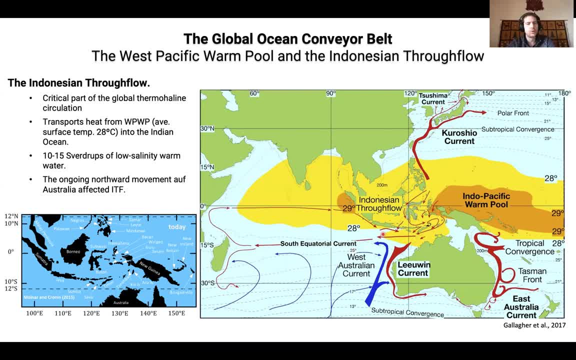 from the Indo-Pacific warm pool into the Indian Ocean, And what is very important about this is the ongoing tectonic restriction of the area because of the continuous northward movement of Australia and its collision with the Eurasian plain in the Indonesian archipelago and on the left hand side. for myself, here you can see the modern 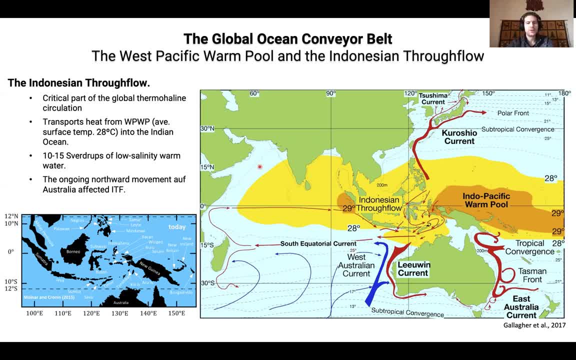 configuration of the islands in Indonesia. but if you look at this in the past, for instance five million years ago, because of this tectonic movement, the configuration of the islands was radically different and a lot of the areas- so everything that is marked in red here- was still submerged at this time. so we have a very clear progression in island uplift. 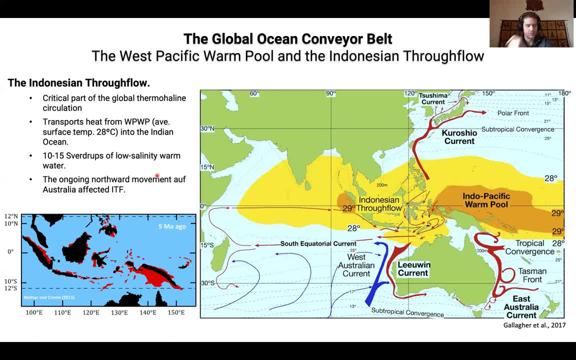 since the last five million years and also in the deeper in the past, but this restriction had then, of course, very likely tremendous effects on how warm water exchange occurred between the pacific ocean and the Indian ocean, and Indonesia expedition 356 had the very direct interest to. 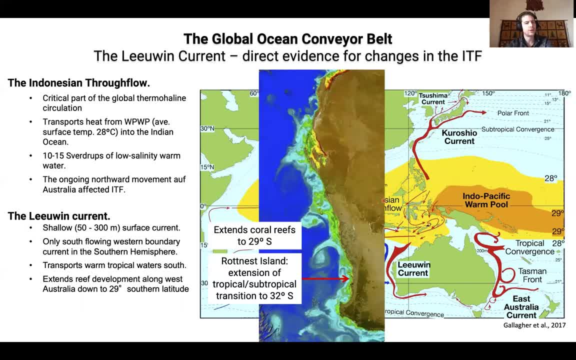 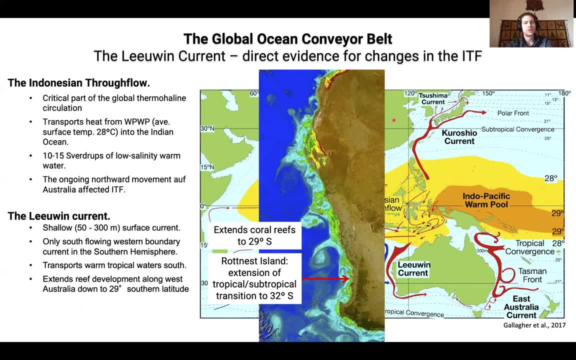 and it is a shallow southward flowing warm water current along the west coast of Australia and it is also the only southward flowing western boundary current in the southern hemisphere which runs basically counter to the general career circulation in the global ocean gyrus and because of that it is a very direct expression of this Indonesian true flow and it is a shallow southward. 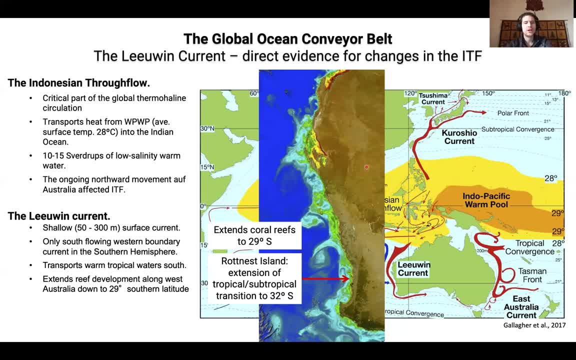 flowing warm water current along the west coast of Australia and it is also the only southward flowing warm water current along the west coast of Australia and it is a very direct expression of this Indonesian true flow. it transports this warm tropical water south. doing this, it extends coral reef up to 29 degrees. 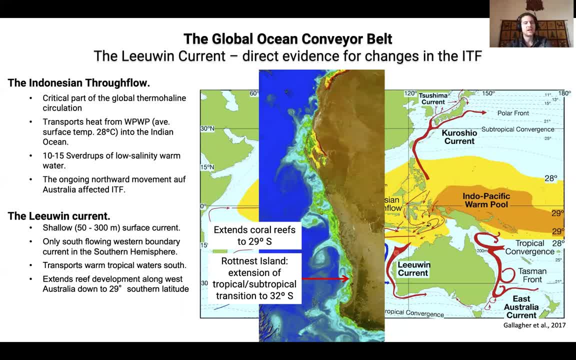 southern latitude along the Australian west coast and it also extends the tropical subtropical transition down to 30 degrees southern latitude. so it has a tremendous effect on the environment of along the west coast of Australia and since it's directly sourced from the Indonesian through flow, it also can act as a tracer. 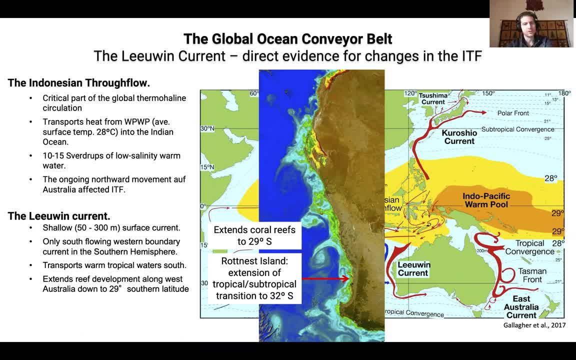 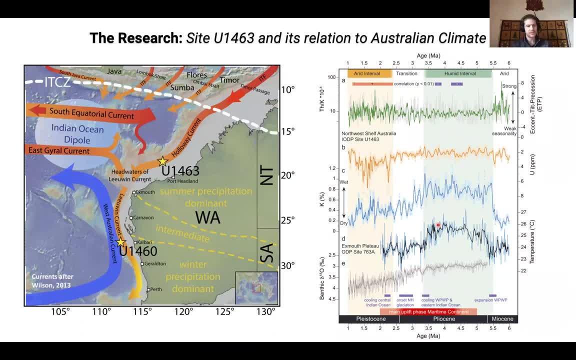 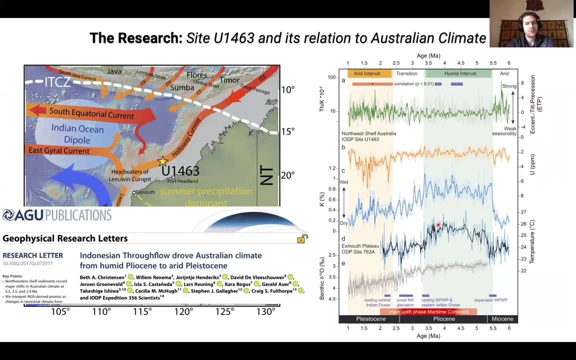 of this ongoing restriction in the Indonesian archipelago directly coming out of expedition 356. one of our first publications that was spearheaded by Beth Christensen, focused on our site U1463, where we analyzed basically the interaction of this proposed Indonesian true flow restriction between five million years and around three million years in the study of Kane and Molnar. 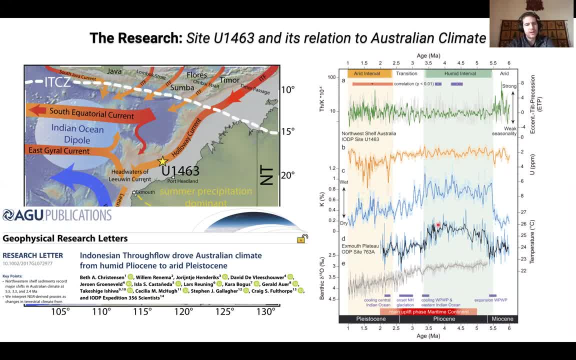 and the beginning, and its interaction with Australian climate. and what we found during this study was actually that Australian climate was heavily dependent on the geometry of the Indonesian food flow and thus also the moisture transport and also the extent of the ITC set during that time. so there is an interaction to the monsoon system in this case and the restriction of the Indonesian 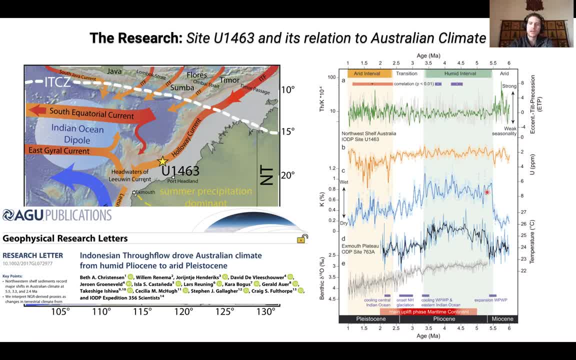 fruit flow apparently moved the Australian climate from the relatively humid conditions in the northern parts of Australia to very dry conditions as we know them today, and this was a very drastic and relatively fast shift that occurred, very similar to other proposed changes that were caused by the direct restriction of this Indonesian free flow around 3.5 to 3 million years. 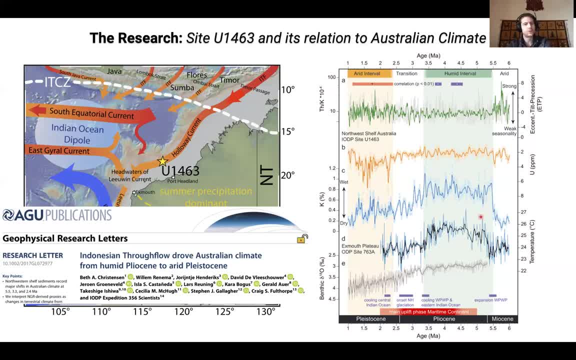 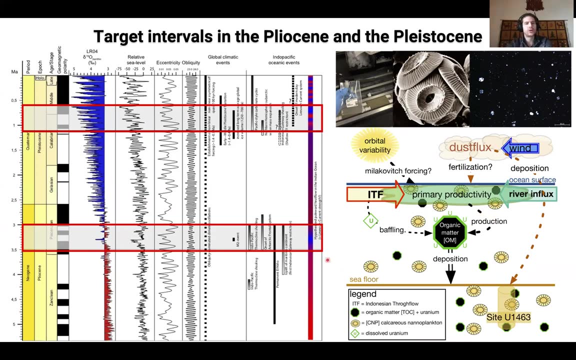 This was a very nice outcome of this research, where we could show that the Indonesian free flow was directly responsible for this and we also had a very nice interaction of this. To further this research, we then moved on to select two target intervals for a more specific 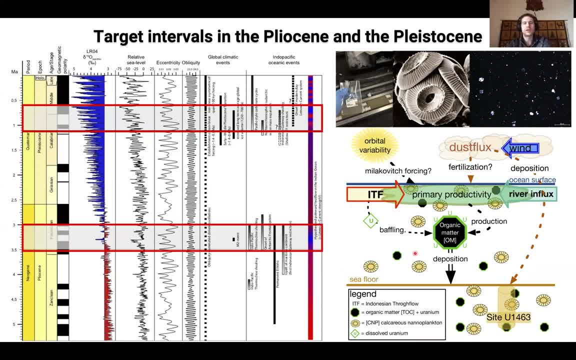 research where we wanted to look at all these processes that we had now on a large geological scales and tectonic scales into sub-Milankovitch scales if possible, but at least on Milankovitch cyclicity, And to study them further and see the direct interaction of Indonesian free flow and maybe 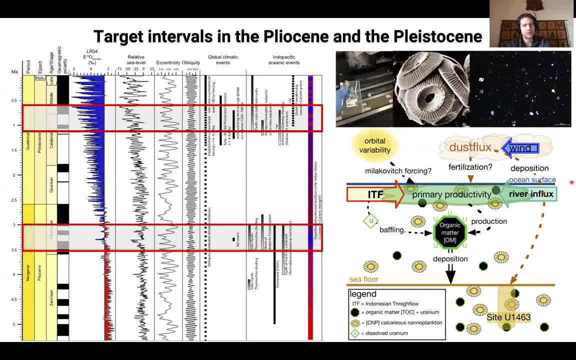 also local environmental conditions, in particular productivity changes and then maybe organic metaflux changes, with different proxies in this case. For this we selected two intervals in the Pliocene and the Pleistocene. One encompasses a 500,000 year interval along the M2 event, which is described as the first. 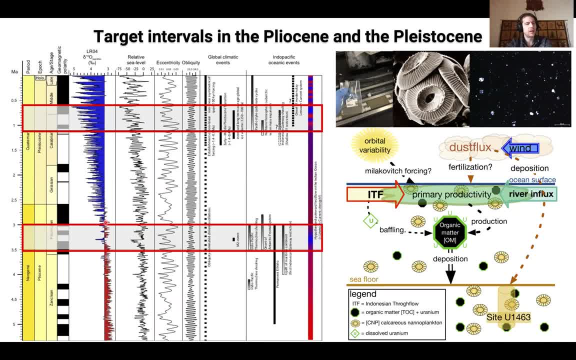 significant glaciation In the Pliocene and sometimes also described as a failed glaciation. it's this tiny little blue blob here which basically shows that it's the first significant cold period in the otherwise relatively warm Pliocene. And the second part which I want to talk about a bit are the significant changes during the 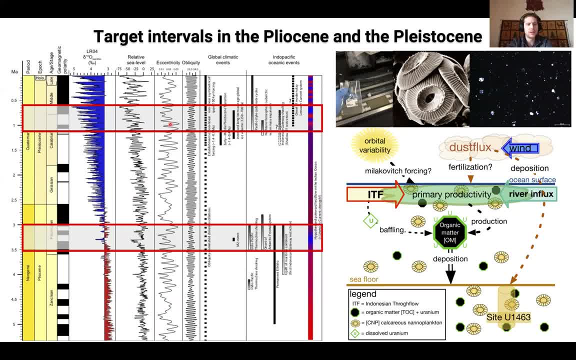 middle Pleistocene transition, which occurred around 1 million years ago, where you have this switch from a dominant obliquity forcing in glacial glaciation. And the third part which I want to talk about is the transition from glacial interglacial cyclicities towards a more or less quasi 100,000 year pacing of our classical Pleistocene glacials. 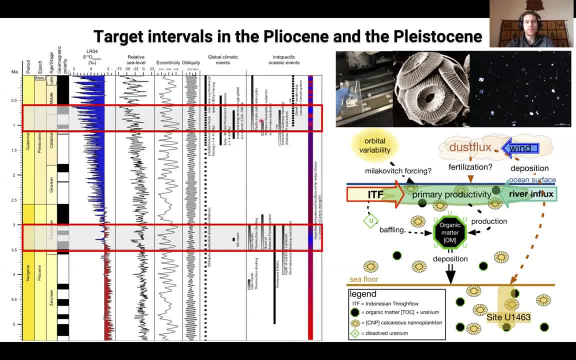 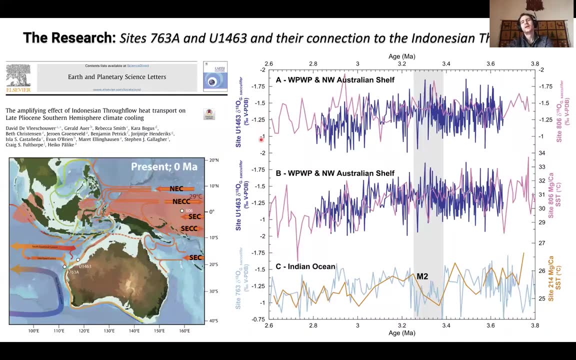 And for this we had a look on our sites and wanted to see the interactions of the Indonesian free flow and also the looming current during these times of significant climatic changes. Oops, are we going? Yes, So the initial study that we had showed actually very nicely that our site U1463 continued. 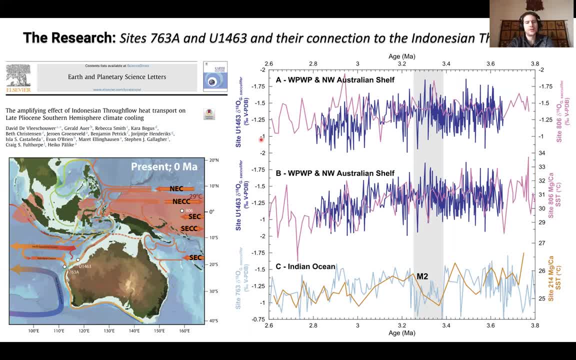 to actually reflect an Indo-Pacific signal, so a West Pacific warm pole signal, during this M2 event, while a very closely adjacent site apparently moved outside the influence of the Indonesian free flow, or the looming current more specifically, and started to reflect the more open Pliocene. 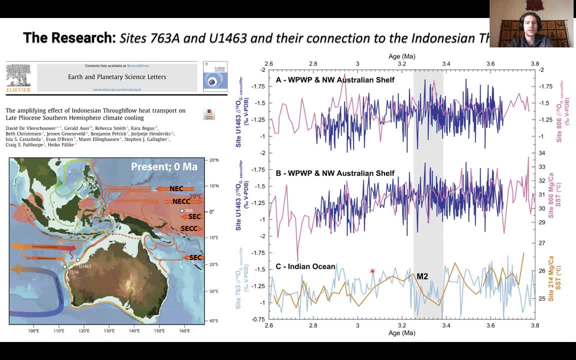 So we had a look on our sites and wanted to see the interactions of the Pliocene and the Indian Ocean signal during the M2 interval during basically this long-term relative glacial low stand between 3.4 and 3.2 million years. 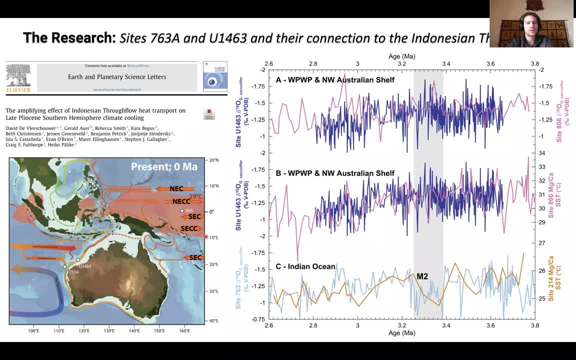 While all our other sites with comparisons from the West Pacific warm pole site here seem to reflect this continuously. So there seems to be a interaction in this that the free flow never specifically ceased or was restricted so much that the environmental conditions Okay Lodging was crossedho听. 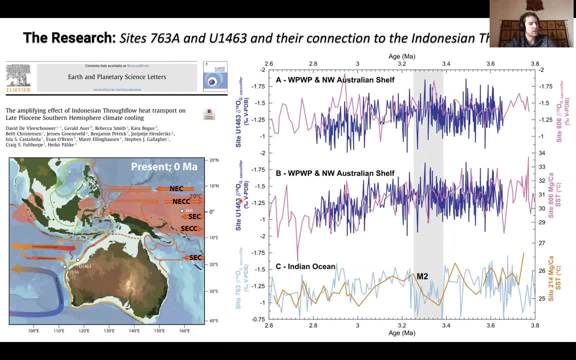 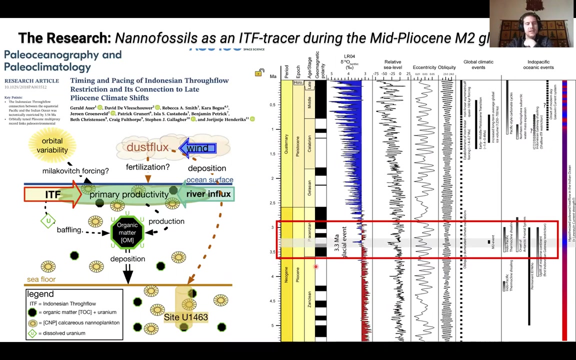 the. So then, the question remained: was this a trickle down effect from an actual tectonic threshold that was reached at some point? Or was this just a classical glacial driven sea level restriction and the reorientation organization of the oceanographic currents around this area? and to better understand this, 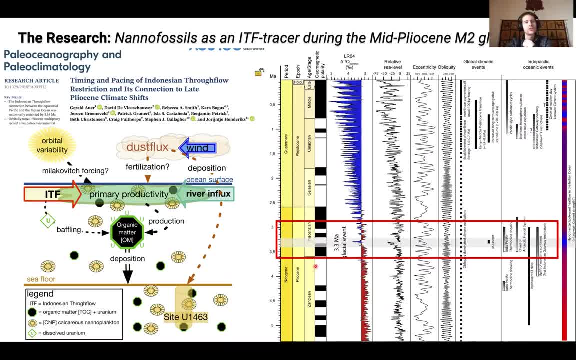 interaction of oceanography. um glacial sea level low stand during the m2 event during around 3.3 million years ago, we started a study that focused on calcareous nanofossils as a tracer for these water masses and their interaction with different productivity proxies. 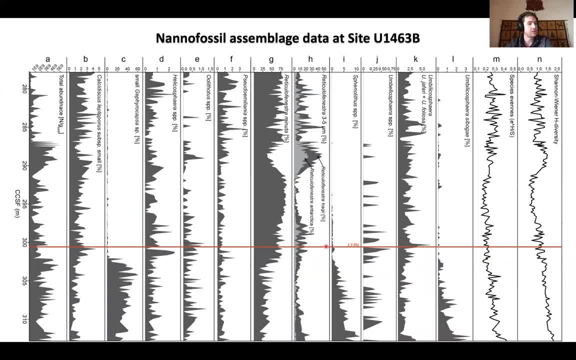 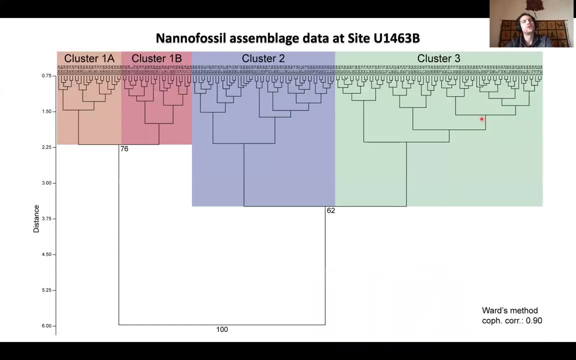 around this time and for this, which, of course, generated a lot of calcareous nanofossil data, which, um in general, looks like this if you have the raw data. i'm not going to go too much into detail about this, because this is usually a huge multivariate data set, but what you can do with. 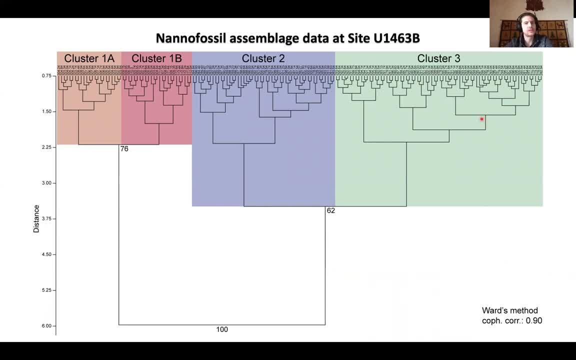 this various nanofossil assemblage status. you can cluster them. so basically, you you bin together samples with similar nanofossil composition and see how they changed in the progression of your sedimentary record, and then also with an age model attached to it in terms of. 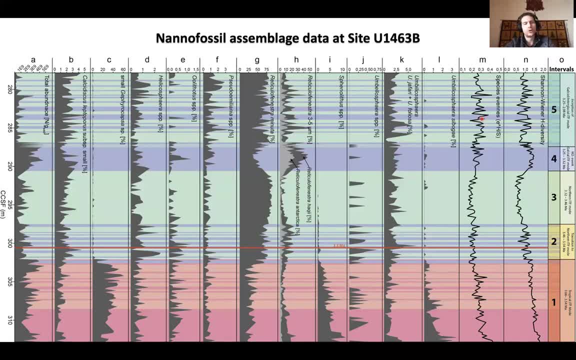 time For this. we then were able to generate various areas of sediment that were affected or basically contained a similar nanofossil community, and this means they also reflect similar environmental conditions. To see this, we basically see a predominantly tropical assemblage in the lower part of our course, then we move to a more transitional assemblage and then we have a 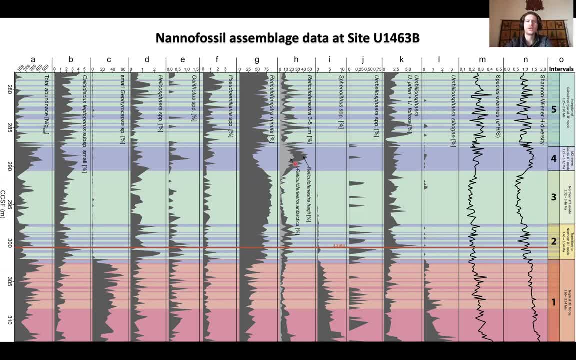 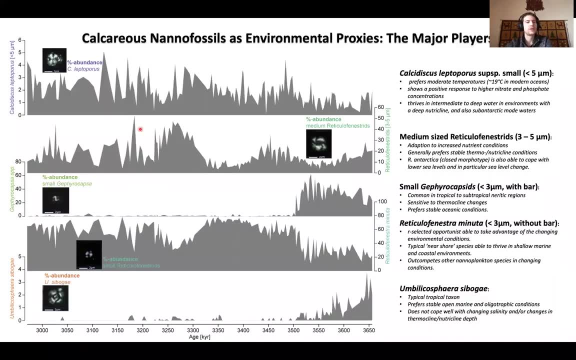 short interval, with a relatively cold assemblage and then a very highly variable assemblage in the highest parts, Continuing this into the age domain. we can then also look at specific so-called index taxa that basically, are major players in the assemblage and that define it. and there we have. 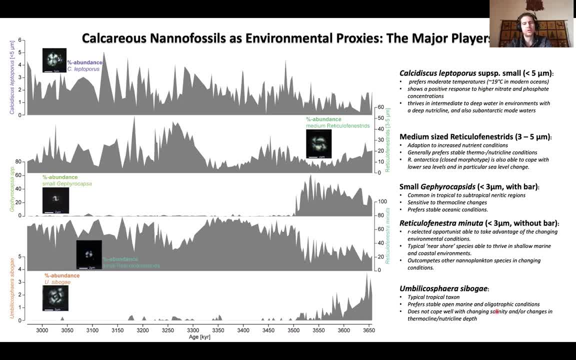 some specific calcareous nanofossils like Umbilicosphera sibogei, which is a very classical tropical calcareous haptophyte that is very indicative of tropical warm water conditions. and then we have very opportunistic taxa, some very near shore taxa of small Cephotocopsids around. 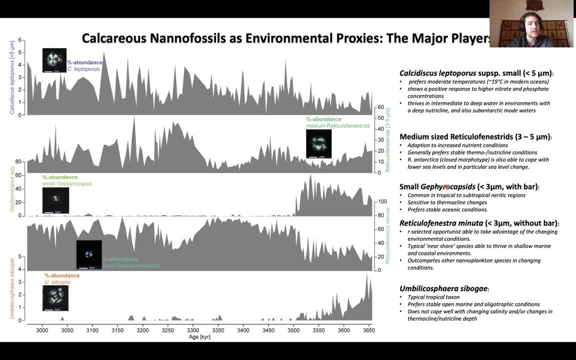 that time that prefer stable environmental conditions and are very sensitive to thermocline changes. Then also we have some other examples of taxa that prefer elevated nutrient conditions or even colder temperatures. So with these changes in the assemblage of these tiny little fossils around a few, 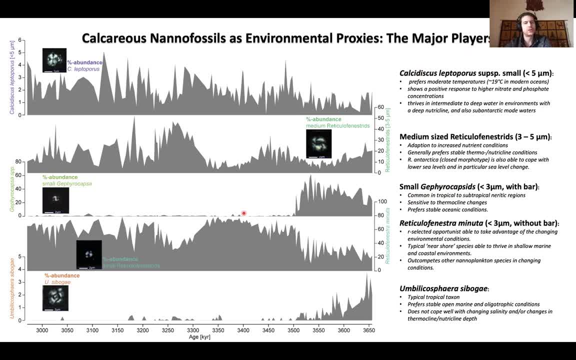 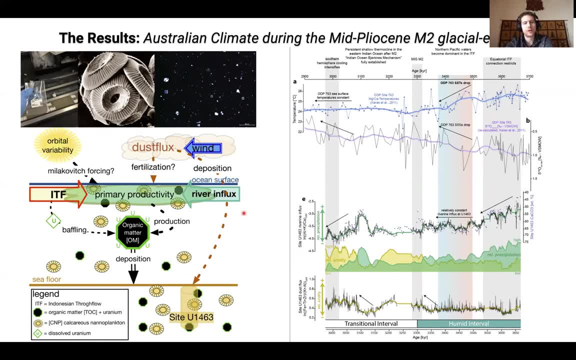 microns only in size. we can then see the change in the class. So here we have a very interesting start to interpret how these changes that we also see in different records that were already published, for instance our humidity record from Australia and also the temperature records from 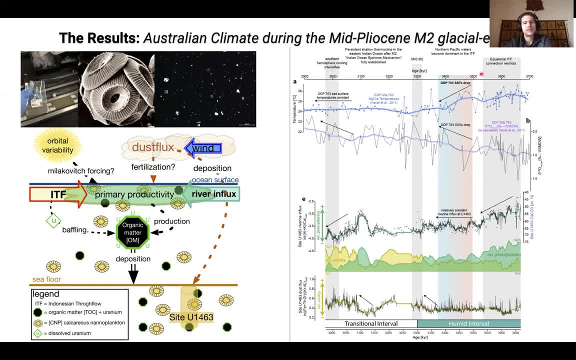 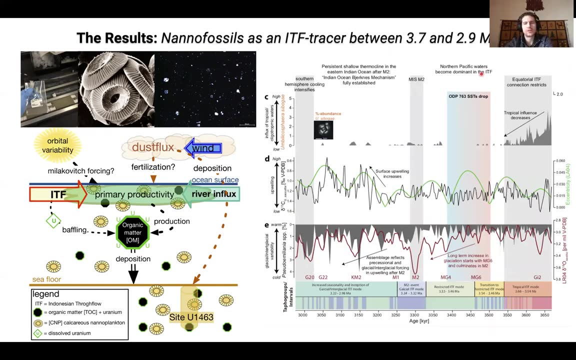 the open Indian Ocean and so how these assemblages interact during this time, and then we can also try and see if there are significant changes that we can ascribe with this, And to do this we combined all our nanofossil assemblage data also with some productivity data. 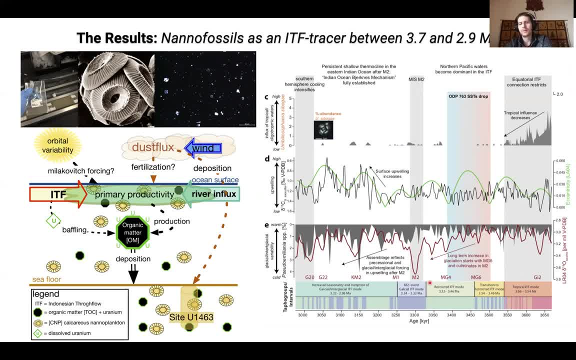 In this case, a colleague of mine contributed the carbon isotope data from Trilobatosaculifer, which is a surface-dwelling planktic ferrominifer, and there we can actually quite nicely see that we see a decreasing tropical influence in the beginning, around 3.54 mSv. 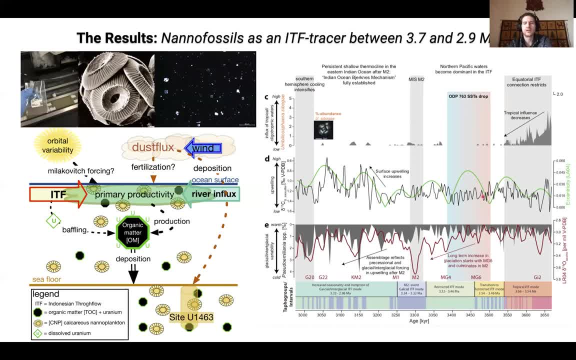 million years. and then we move into a more transitional assemblage and we have the M2 event very nicely recorded also in our nanofossil assemblages down here. And then also we have this very variable post-M2 glacial interglacial cyclicity, where also 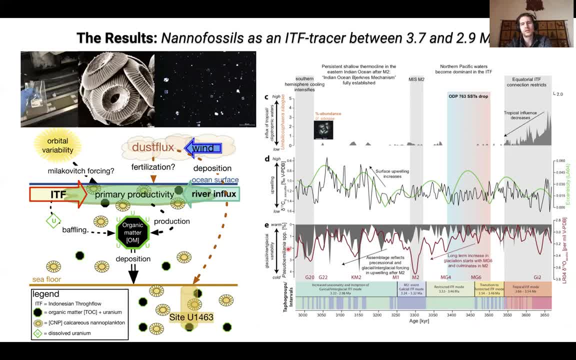 a specific nanofossil taxon follows the global deep water isotope curve of the Liseki and Raymo, the LRO4, quite nicely, And during this time we also see an increase in surface upwelling and thus productivity, which is also reflected in our carbon isotope signatures. quite nicely. 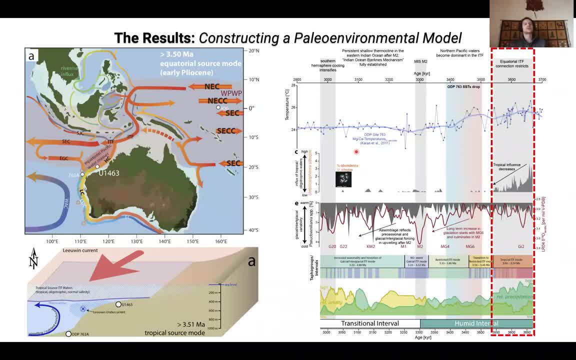 And so, with these changes combined, we can then also start thinking about the tectonic interactions and the global climatic interactions during this time, And for this we basically started a reconstruction of the paleoenvolvement, and for this we also went back to the reconstruction of Canaan-Molnar and the 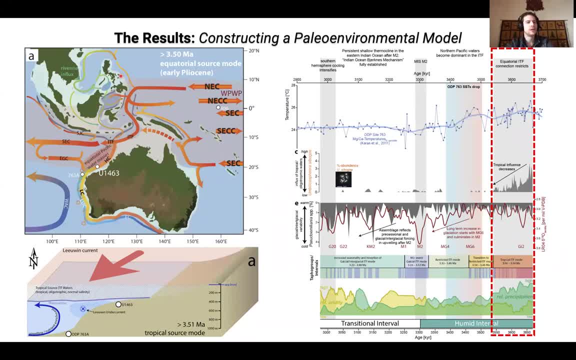 potential emergence of different islands in the Indonesian archipelago and how they might have effect that the Indonesian throughflow around this time. So in the beginning we had the decreasing tropical influence and in our model this basically relates to a very strong, very tropical connection. 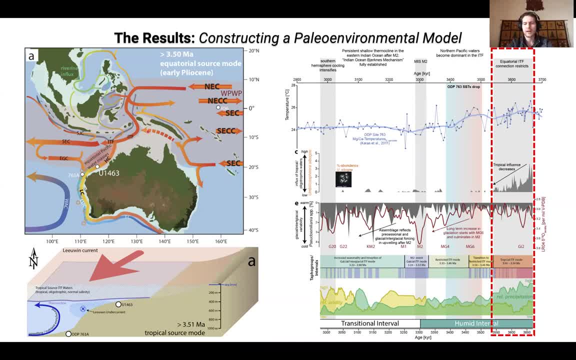 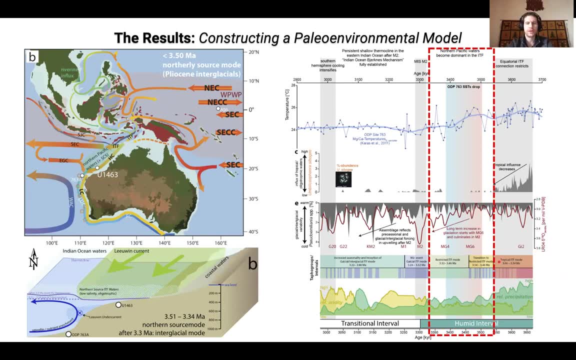 that was still active around the that time And then a certain threshold was ceased where we moved into this first transitional period where we had a very strong nanofossil shift and also the end of the decreasing precipitation in Australia, And we interpret this as a 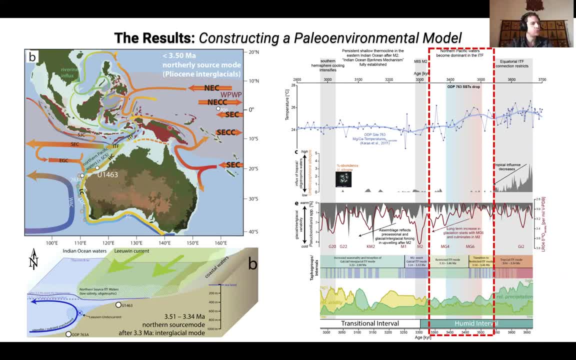 threshold where at least several islands were high enough to limit the moisture transport from the ITC set directly into the northern part of Australia, although some were still continuing. But the most important thing around this time, we consider that around 3.5 million years ago, 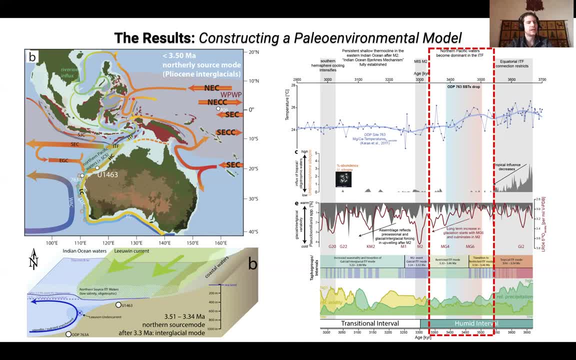 a threshold must have been reached where more than enough islands were uplifted around this time to have a significant source shift in terms of waters that go through the Indonesian throughflow, where we basically propose a northward shift to less saline and less tropical waters. arriving there, They're still very warm, of course, so still tropical to slightly subtropical at most, but there was a 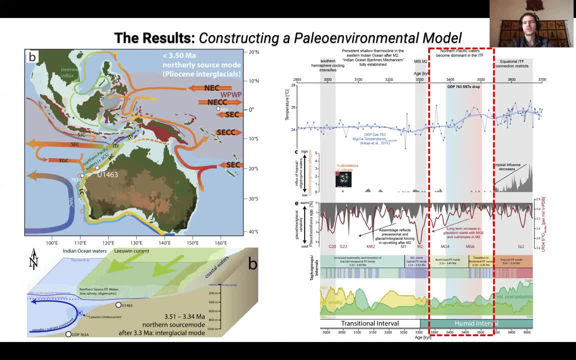 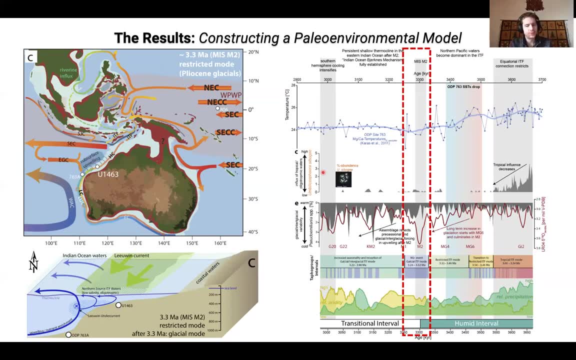 significant shift in the water masses that was recorded by our nanofossil assemblages. The next piece that we found is that the M2 event, as was also previously proposed by our first study that focused on this time interval that the sea level low stand during. 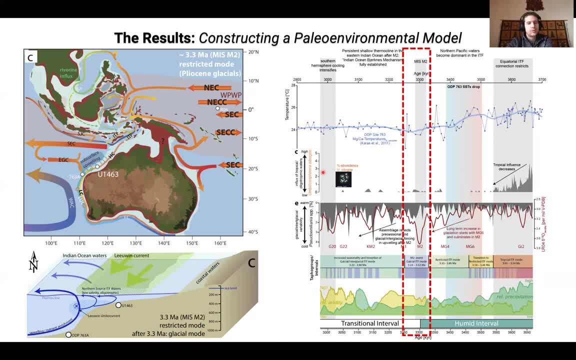 this first significant glaciation, the so-called M2 event, around 3.3 million years ago, further significantly changed the throughflow mechanism, and this was mainly a sea level control and not necessarily a direct tectonic control, Although, of course, the ongoing tectonic restriction only made it possible that sea level. 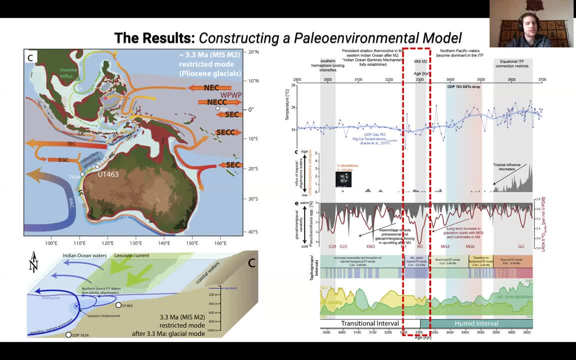 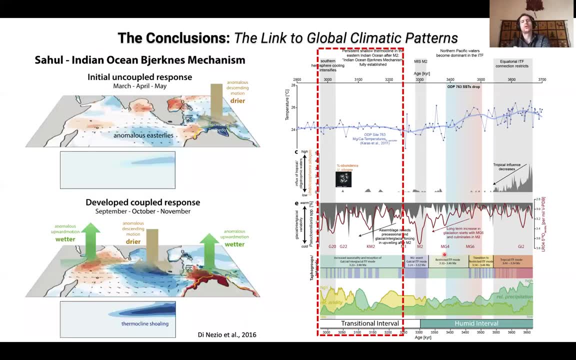 falls managed to restrict dishes as much as they did, And this was also the inception of a very closely ongoing glacial interglacial cyclicity around this time. that is also very well recorded after the M2 event, And so our thinking in this regard is that this. 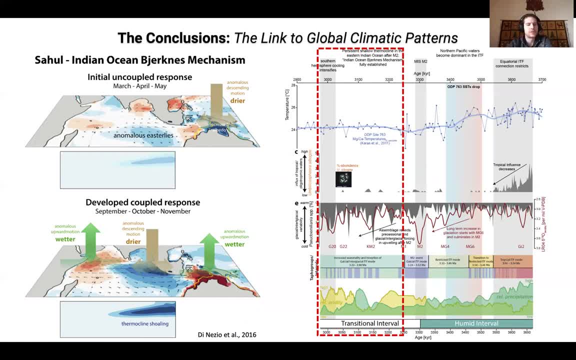 pliocene change was directly responsible because we had continuous uplift of these areas, So the shelf areas increased And during glacial low stance, more shelf areas were exposed during this time And this favored the so-called Sahul Indian Ocean Bjerkenes mechanism, which is basically 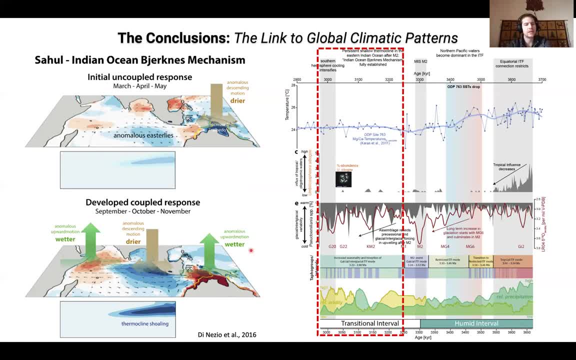 and very simply described a miniscule, mini El Niño system that can establish in the Indian Ocean and thus generates anomalous wind system during glacial low stance that favor upwelling along the west coast of Australia in the eastern Indian Ocean, And so we see this progressive increase during beginning sea level. 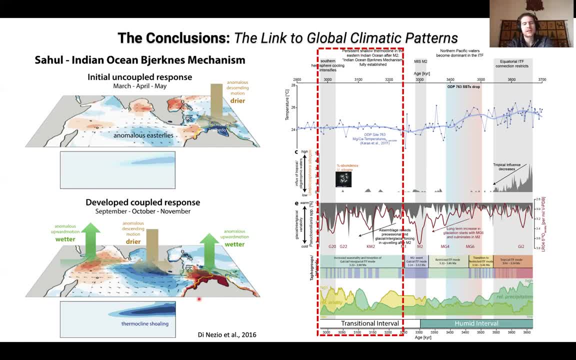 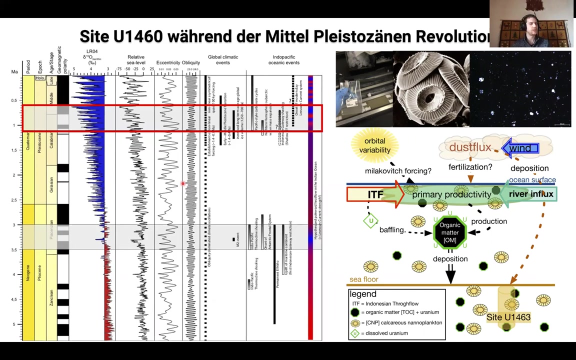 variability. that was increased after this first glaciation, the so-called M2 event, And there we really see a very interesting progression of the climatic interactions based on this tectonic and sea level driven changes during the pliocene Good. This more or less concludes our first foray into the pliocene and showing this very nice. 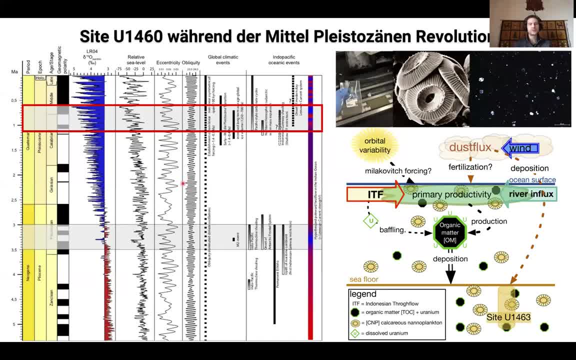 progression of tectonic induced changes that are then amplified by beginning glacial interglacial variability and showing this very nice progression of tectonic induced changes that are then amplified by beginning glacial interglacial variability Following this first initial glacial during the M2 event. 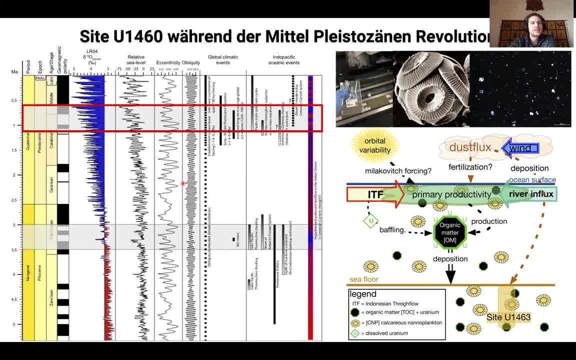 Our next interest was then, of course, the so-called middle Pleistocene revolution, And in this case we have a look at the time until war, from around 1.1 million years to 0.6 million years in the past, where this very strong shift from the 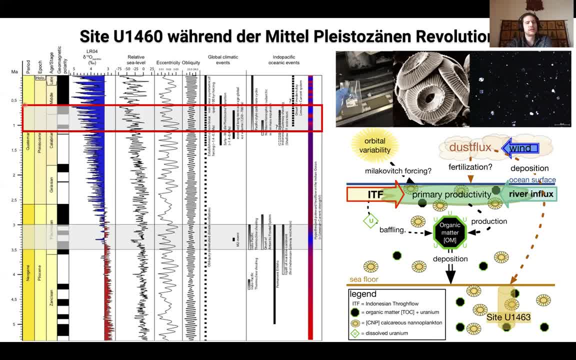 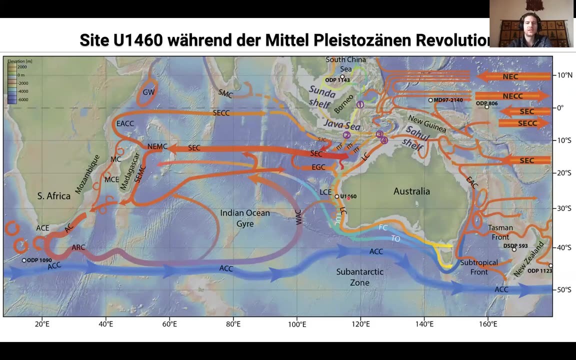 41,000-year obliquely dominated glacial interglacial cyclicity that was persistent beginning with the M2 event in all global records to this quasi-periodic 100,000-year cyclic changes. For this study we moved to site U1460,, which is a bit further south. 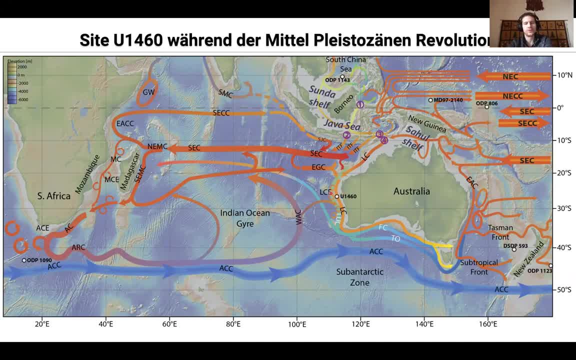 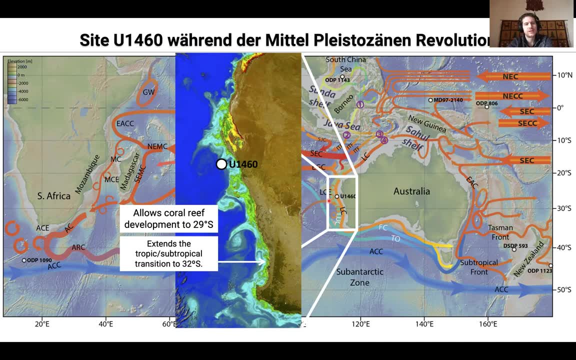 along the western shelf of Australia. U1460 is insofar also very interesting because this site is directly into the path of the Lubin current, which you can see here quite nicely in the chlorophyll data on the satellite image. Everything that's basically greenish to turquoise. 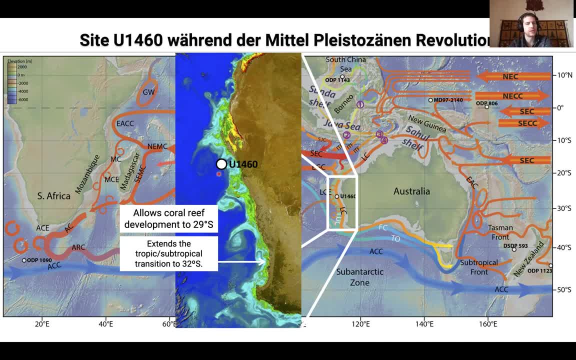 in this image is the Lubin current that affects the productivity around this area. U1460 sits right at the edges of this interval and so any kind of changes that affect the shelf areas during glacial, interglacial cyclicities, and also changing the strength or position or 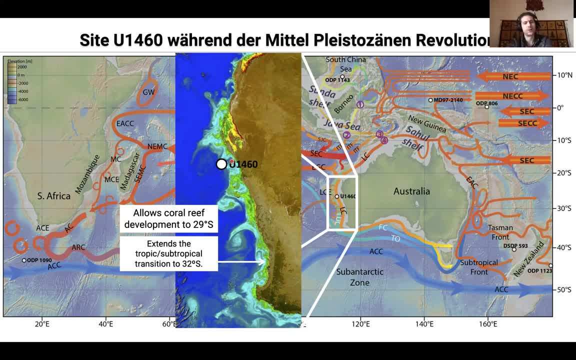 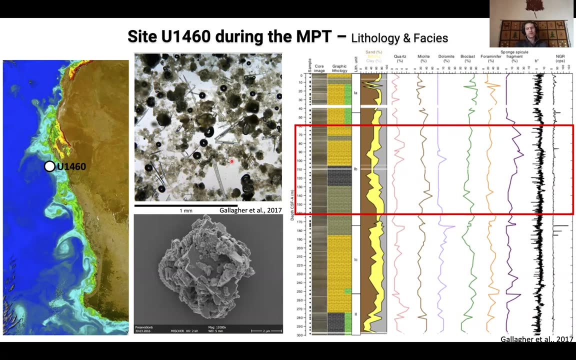 turbulence of the Lubin current in this case might also heavily affect U1460 in this case. We also selected a sampling interval at this second site that we studied in this case. U1460 has, for one thing, a very interesting paleo oceanographic potential in this case, but it also has a very interesting sedimentological 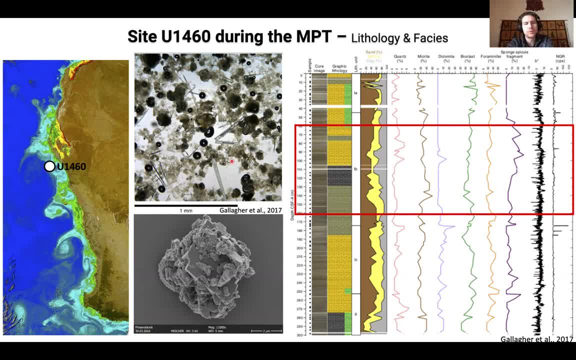 composition in this case, because it is a very shallow marine site where we also have proto-dolomite formation. We have a basic sponge reef that we drilled into of eugenic gluconide formation, So there's also a lot of sedimentary and also early. 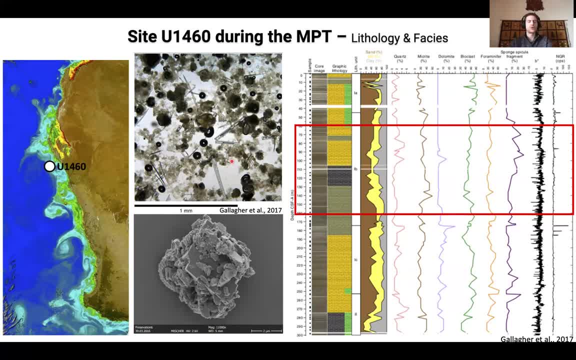 diagenetic interactions, which we will also currently studying, And this is so ongoing research processes that we are currently invested in. But, for this current example, we are in the beginning only focusing on the paleoenvironmental implications of the sea level changes during the 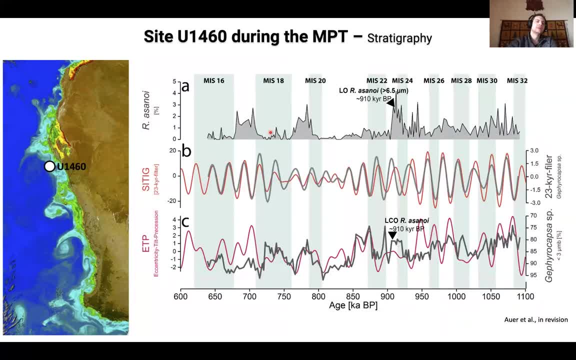 MPT For this. of course, the first and foremost important thing for analyzing and studying such changes in the past. a proper and verifiable age model is, of course, the most important thing For this. we again used calcareous nanofossil as a primary biostratigraphic marker. Here I just show the 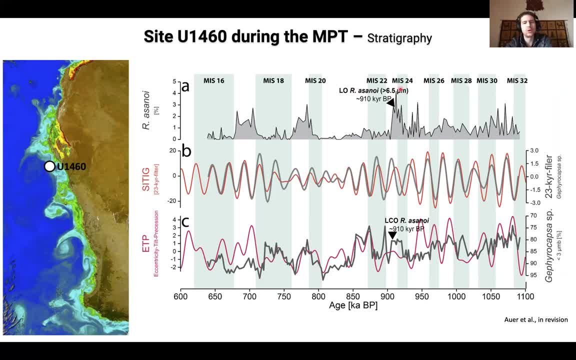 last occurrence of larger reticulofenestra esanoi, which, in this case, we took as a marker for the last occurrence, which should have globally occurred around 910,000 years in the past, And using this age model combined with shipboard biostratigraphic data, which is also based on: 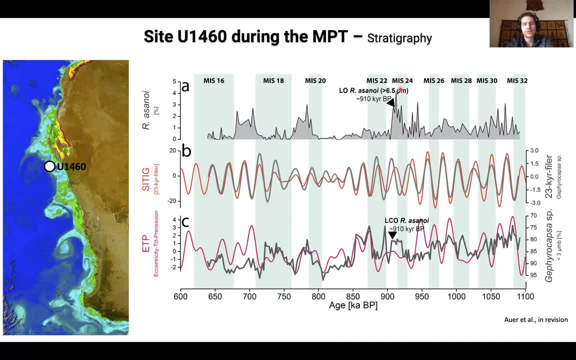 calcareous nanofossils and planktonic foraminifers. we were able to generate an orbitally tuned age model which in this case, focuses on the changes also in the nanofossil assemblage, In this case the variability of small gefürokapsa in the record. 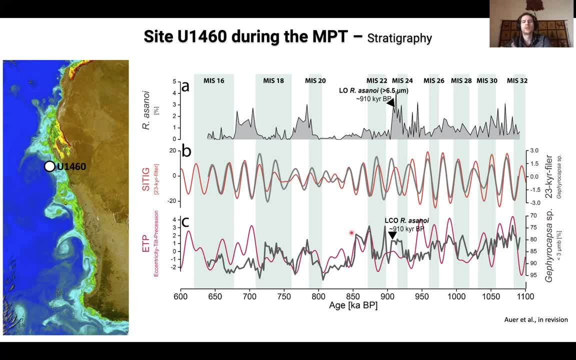 And, as you can see here, there's a very clear orbitally paced variability in these abundances, which are basically related to the light intensity, the variability of the ITC set and thus also, in part, the monsoonal variability that affect the northern parts. 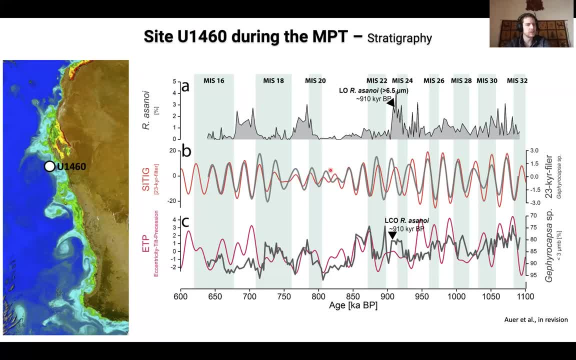 of Australia, with the Australian summer monsoon in this case, And using this interaction, we were able to orbitally tune our depth-based data from the IODP course and then also interpret them in terms of time over the MPT interval between 1.1 and 0.6 million years in the past. 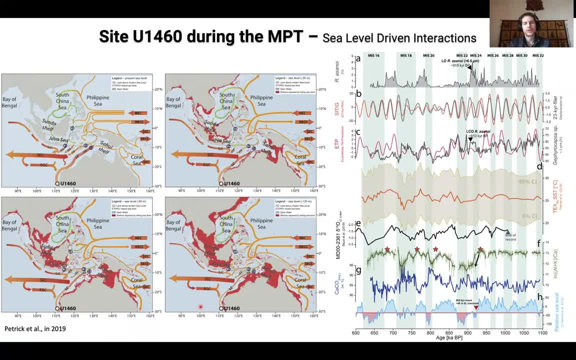 The first thing that we noticed during this study was that there was a heavy effect of sea level driven changes that began to amplify after the so-called 900 kilo year event, which is marked in this unfortunately rather small figure here, Beginning with a dramatic sea level low stand of 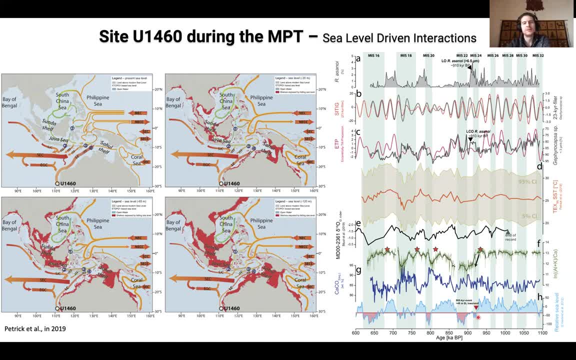 around 45 meters below present, which was very much a first threshold that began to affect this relatively shallow site. As a very important mention, U1460 lies currently only in 240 meters of water depth, So any kind of sea level changes of course dramatically affect the environment on the shelf that is recorded at. 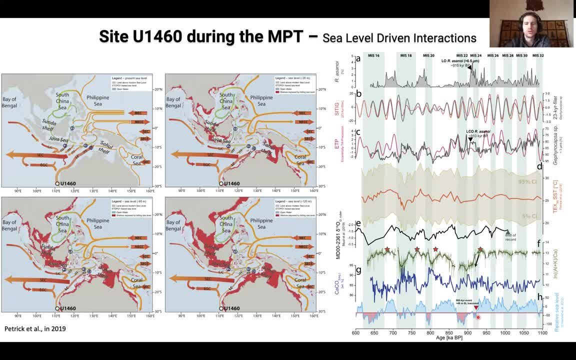 this one position where the site was drilled. And so, with this one sea level change, we very curiously detected an increase in carbonates during sea level low stands that fall below 45 meters, which you then interpret to a shift to more benthic, dominated shelf productivity. So we basically move. 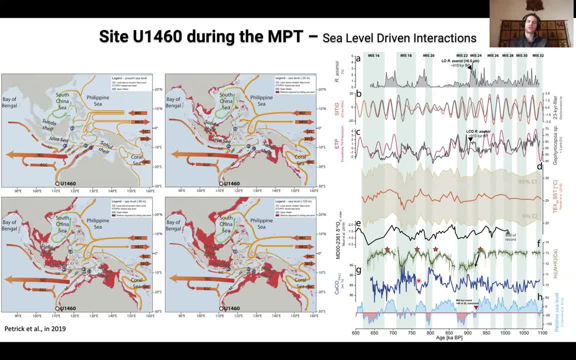 from a more open marine outer shelf environment that is, more pelagic productivity dominated, to a more benthic productivity dominated, setting around this time when there is sea level low stands And this very strictly tends to affect also the carbonate concentration, because there's basically more 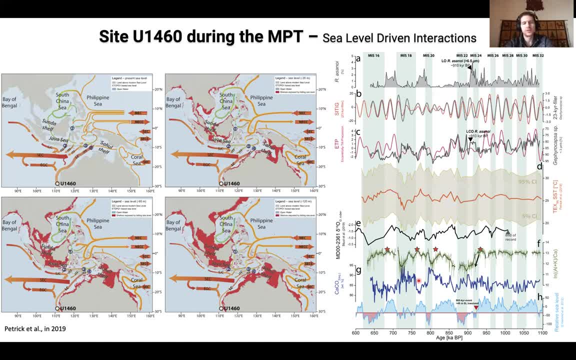 benthic organisms that gets transported here, So larger benthic foraminifers, various bivalves and gastropods that just generally predominantly accumulate during the glacial low stands. This is also reflected in our surface water temperatures that were donated by Ben Petricht and Alfredo Matias-Cassia. This is also reflected in our surface water temperatures that were donated by Ben Petrich and Alfredo Matias-Cassia. This is also reflected in our surface water temperatures that were donated by Ben Petrich and Alfredo Matias-Cassia. 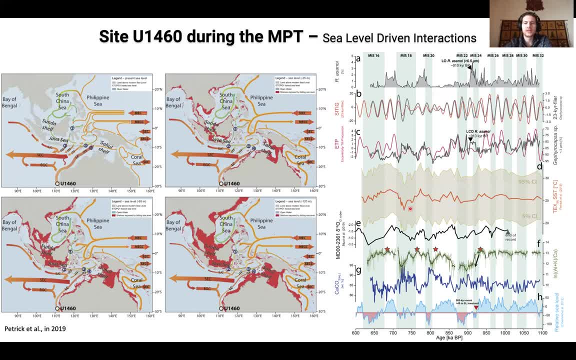 This is also reflected in our surface water temperatures that were donated by Ben Petrich and Alfredo Matias-Cassia In this comparison, and there we actually see that we also increase the glacial interglacial variability in temperature drops following this MPT event. 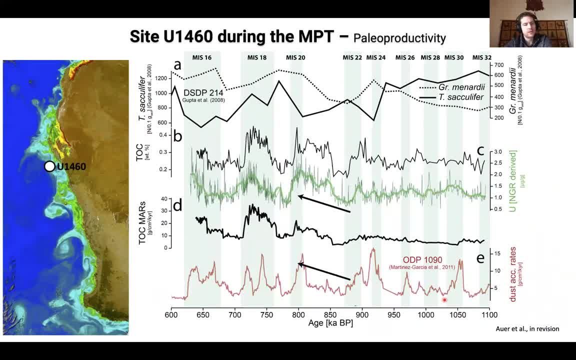 And what we were primarily interested in this study was, of course, the effect of the sea level changes on the lubin current directly, And for this we were specifically looking at various paleoproductivity records in the past that tended to affect the site U1460 during this time. 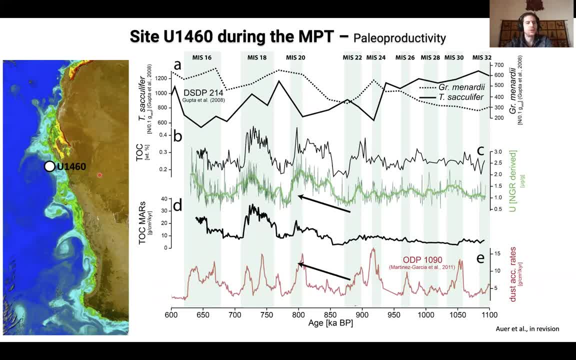 Paleoproductivity is a very interesting tracer for the lubin current because of course it is a warm, oligotrophic current that flows down, So any kind of changes in the strength of this current will also directly affect the nutrient conditions. This means the less intense. 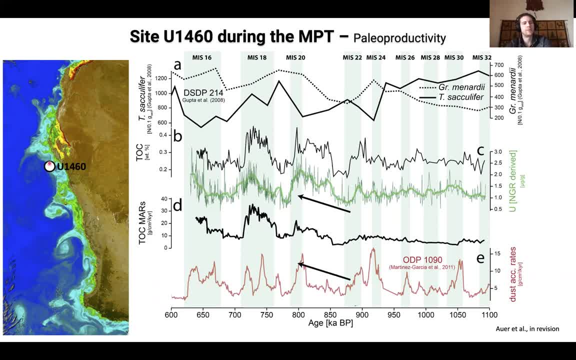 the current gets, the more likely it is that classical upwelling through Ekman transport gets increased at U1460, thus potentially also increasing deproductivity around this time. And to see these changes, we focused on organic matter accumulation rates and also our uranium. 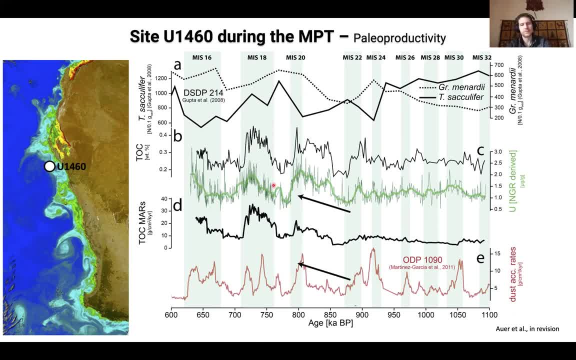 content as an additional independent proxy, Because uranium is, of course, directly related to organic matter through a complex process of complexation in the water column, where basically uranium tends to bond with dissolved particulate organic matter. that then gets transported into the sediment and preserved during various mineral phases. 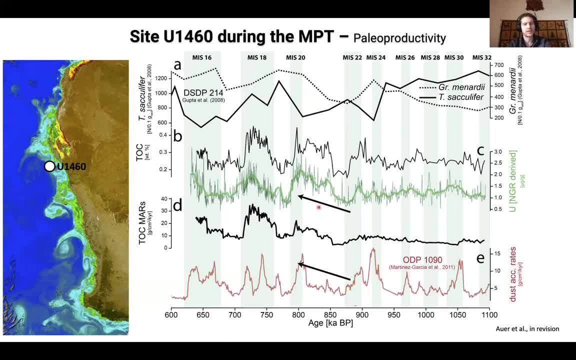 And what was very curious to us is that before this 900 kilo year went, so before this first dramatic sea level drops around 900,000 years, productivity around the west coast of Australia was relatively stable and very low. So in our understanding this means that there was a very constant and warm lubin current still affecting 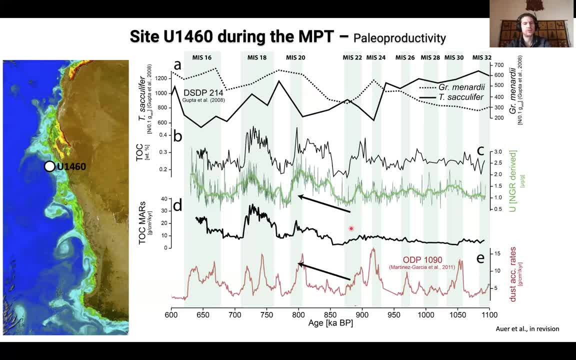 this site. But as soon as the sea level drop occurred a very strong shift and an increase in productivity occurred after the sea level bounced back. So we saw we see a complete shift in how the environment responds following this 900 kilo year event. sea level low stand. 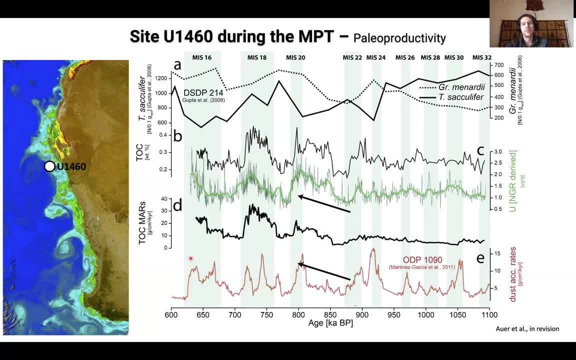 And to show that this is apparently relatively unrelated to the global productivity records in glacial interglacial variability during the mid Pleistocene. we also plotted the Southern Ocean dust flux from ODP 1090 here, which basically reflects iron fertilization in the 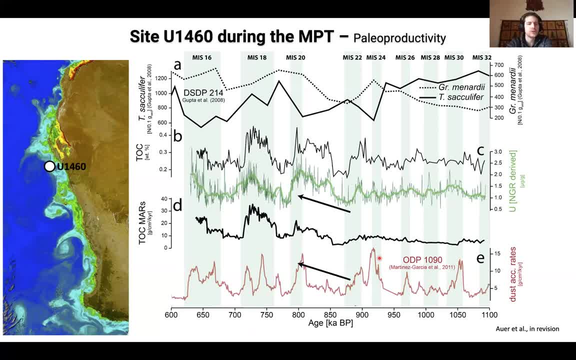 Southern Ocean sector Of the world's ocean And there we see that basically organic metapherial is not directly paced with these global dust records but it is a very much local and maybe directly shelf signal that we can see here And this is potentially very much reflected to different 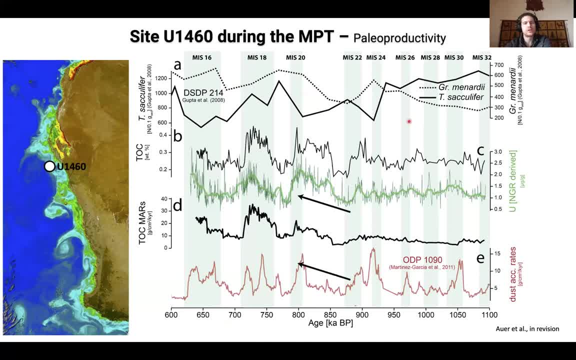 changes in surface water conditions around this time, which we can also see in different sites. This is a tropical site, the SDP 214, which lies on the 90 Eastridge in the Indian Ocean, And there we also see very strong 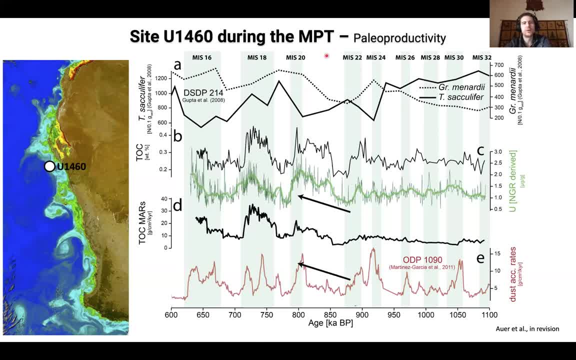 thermal client changes during MIS 24 to MIS 22.. So directly during the MPT and the 900 kilo year event, And in our interpretation this is a permanent increase in thermal client tilting around this time, which then also favors upwelling and also the 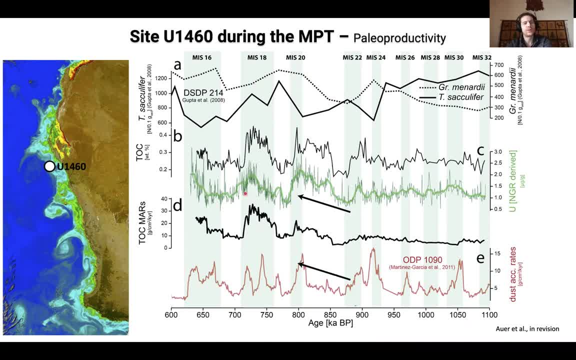 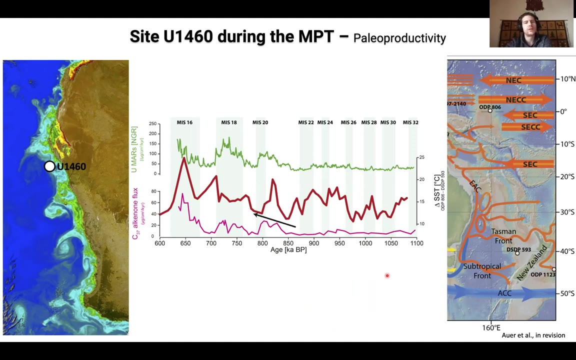 transport of nutrients to the surface for various eddy mixing, which also occurs during times when the lubin current is stronger in interglacials, And this specifically occurred after the 900 kilo year event, And this increase in productivity is also related to an increase in basically hemispheric 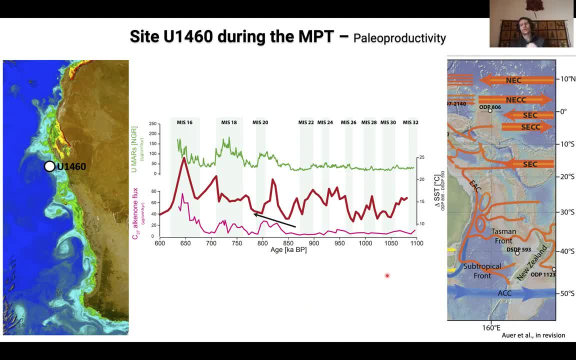 temperature gradients, Meaning the stronger gradients between the tropics and the high latitudes in the southern hemisphere became following the 900 kilo year event, the stronger our productivity records become, And this is not directly and easily interpretable with our data and our understanding of how the interaction of the local 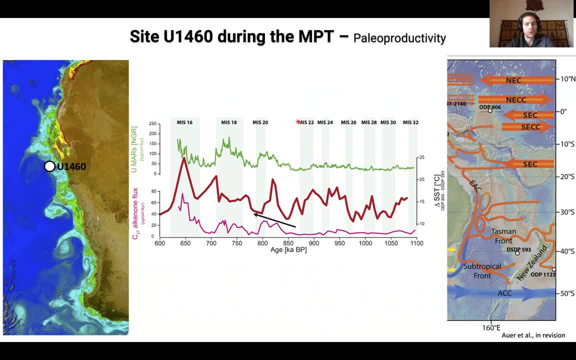 of the lewin current should work during glacial interglacial periods. so basically you have a reduced lewin current because of glacial low stance and thus a reduced through flow through the indonesian archipelago. so there might also be a different transport mechanism of general. 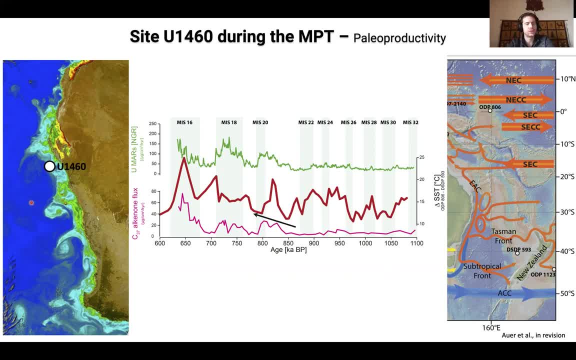 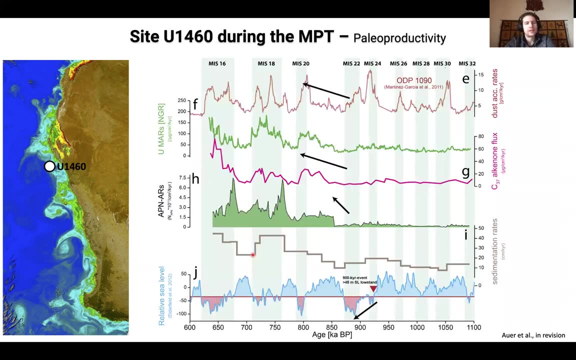 nutrients that might have reached u1460 following the mpt event, and this is something that we then also would have wanted to have a look at and, beginning to unpuzzle this um we were able to actually um look at productivity, um variabilities in direct contrast with our nanofossil accumulation rates. 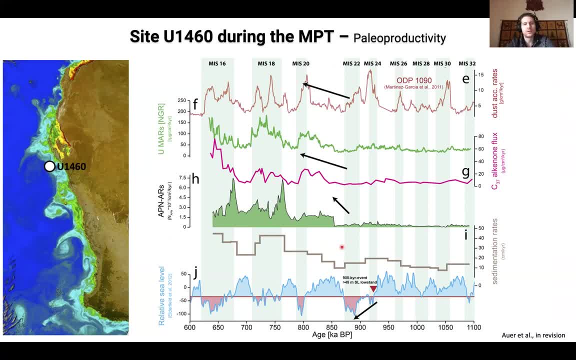 which we see here in this solid green graph and where we see that there's a definite increase following the 900 kilo event here, where we then have a increase in nanofossil accumulation rates and general productivity during the next sea level high stand and this means that there is a significant shift in nutrient availability. 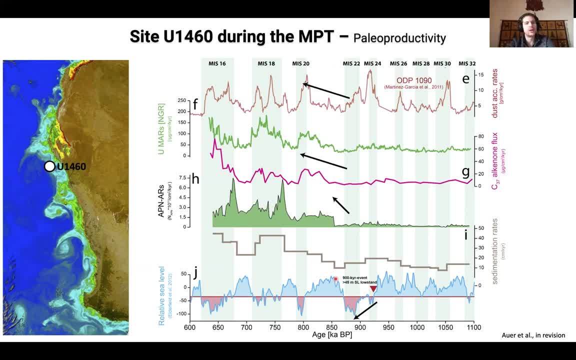 following the 900 kilo year event, and then also an associated return to more open marine and planktic production, with which that of course equates to the increase of the range of the, the walkway and, uh, the cold water transport system, which is the on the left and the one at the bottom. 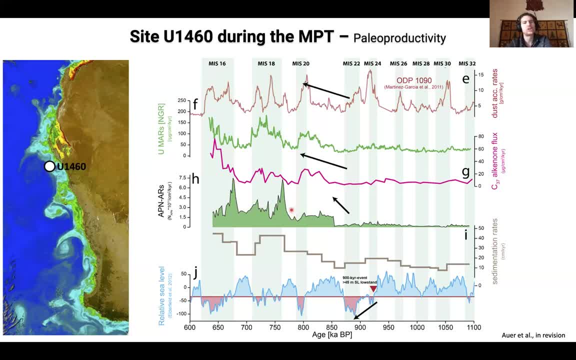 and the all the way down to the bottom of the ice romeo, and also the comparison with the this productivity record. but they do show spikes following the highest sea levels during interglacial, beginning at the interglacial towards glacial transition, where they show. 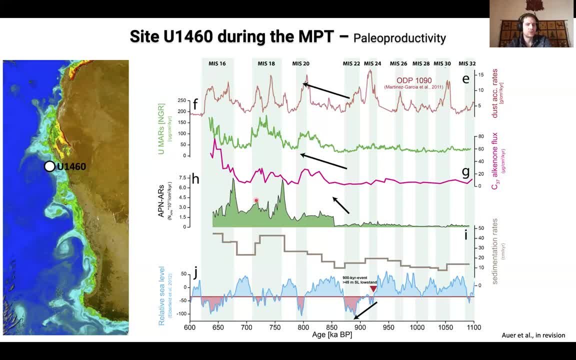 our highest abundances And this was very interesting to us, and we do interpret this as a highly eddy-dominated regime around diluent current system which transports nutrients in a still relatively open ocean system which favors the accumulation of calcareous nanofossils. 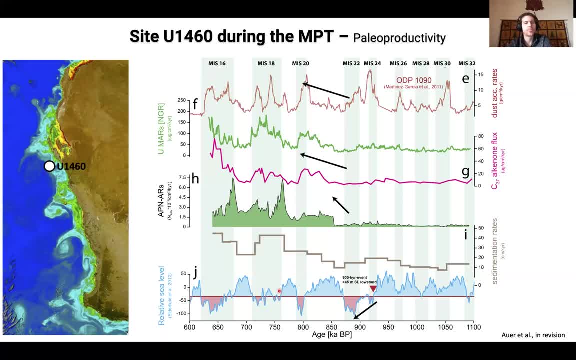 And later on, when sea level drops further. productivity continues to be relatively high for different upwelling processes in the surface ocean, But this is then dominated no longer by classic open marine calcareous nanofossils that generate the alkenones, but also through coastal species. 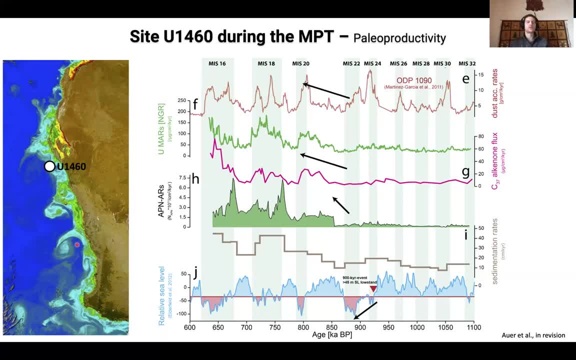 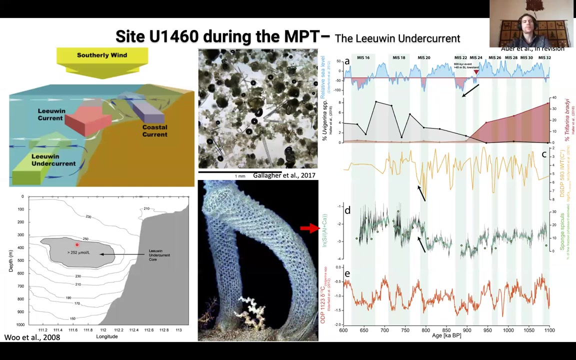 So there's also, then, Again, an interaction of lubin, current strength, different sea level interactions and also the local environmental conditions that we then have recorded in our site directly And to further study this, and this is currently an ongoing research topic for us. we began 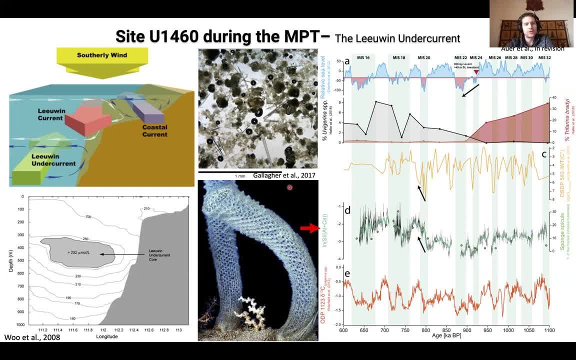 to think how nutrients would actually arrive at the site, Because, even though there is upwelling, you also need to have a relatively nutrient-enriched, lower thermocline or lower thermocline waters that have to transport the nutrients at the site. U1460, actually. 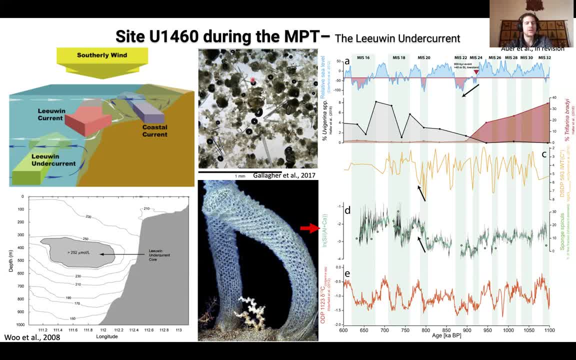 And what was quite interesting at site U1460 is that we drilled. a lot of sponge remains in this case and sometimes we actually found in-situ sponges. So we drilled into a A sponge reef that occurred around the shelf areas, around 200 meters water depth in this. 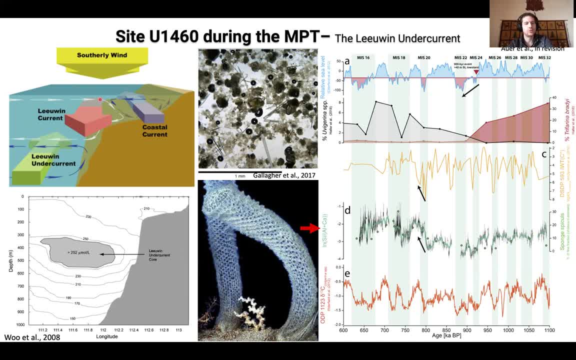 interval that was otherwise surface water influenced by the lubin current, And so this means in the lower area there had to be relatively cold, a relatively cold current that established around sometime that favored the growth and establishment of various sponges in the area. 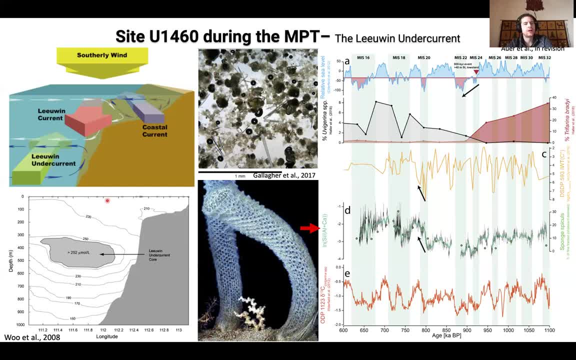 And looking at the oceanographic conditions here, Below the lubin current there is the so-called lubin undercurrent, which is a northward-flowing countercurrent below the lubin current, which transports relatively oxygen-rich cold waters from the subtropical and even sub-winter arctic transition zones south of Australia northwards. 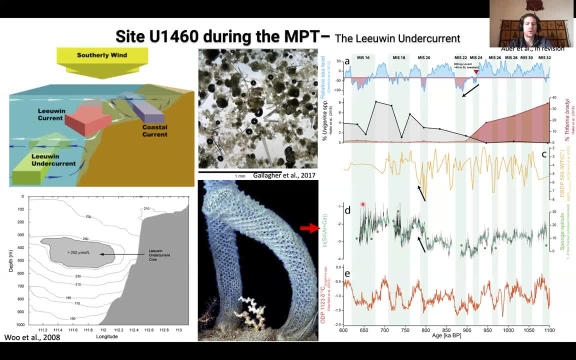 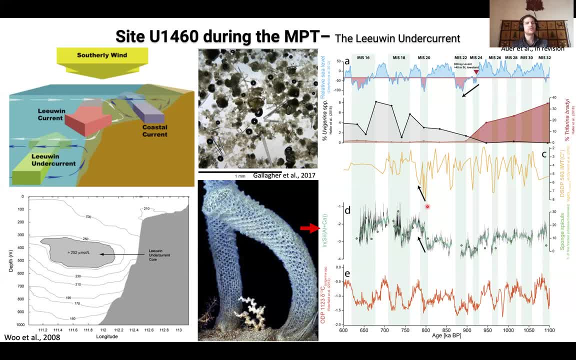 We then also relate to maybe a shift in the nutrient transport and potentially also the strength of this undercurrent, And this is also well reflected in our understanding of the preliminary benthic foraminiferidator that you can see up here, that we are currently in process of generating with a PhD student. 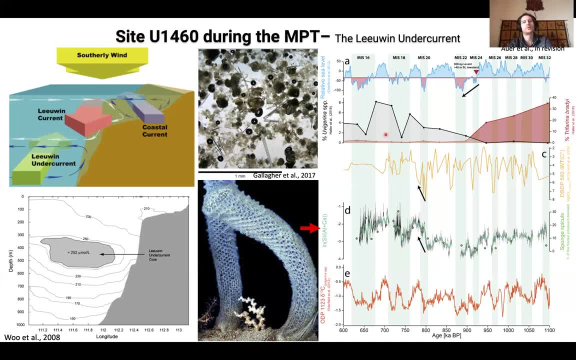 of mine Where you see a very strong shift between between detritus feeding planktonic foraminifera following the NPT event versus lower infonol and also facultative anaerobic planktonic benthic foraminifera. I'm sorry, benthic. 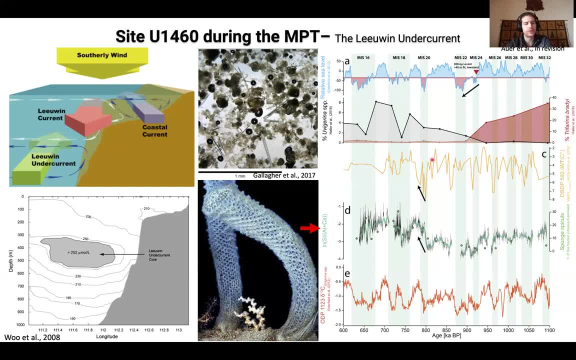 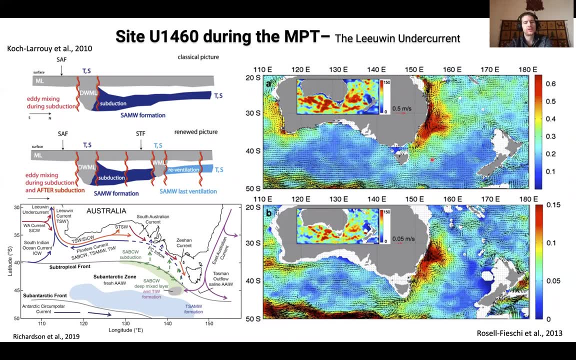 foraminifera before the NPT event. So there seems to be also a very strong change in this undercurrent And the understanding how this undercurrent changes might be related to the NPT in general can be explained if you look at the oceanography of the Australian sector, so the South Australian. 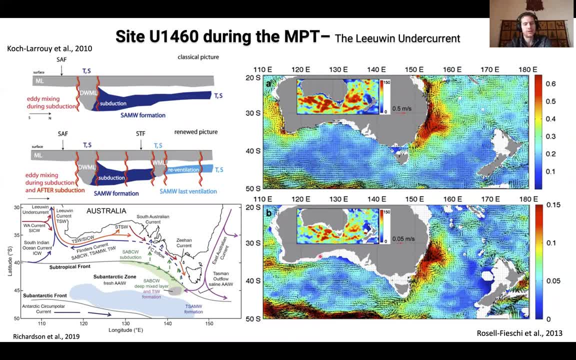 sector around the Great Bight of Australia down here south, because this is one of the formation regions of so-called sub-Antarctic moat water In the Indian Ocean. This water is basically relatively cold water that subducts in the deep winter mixed layers. 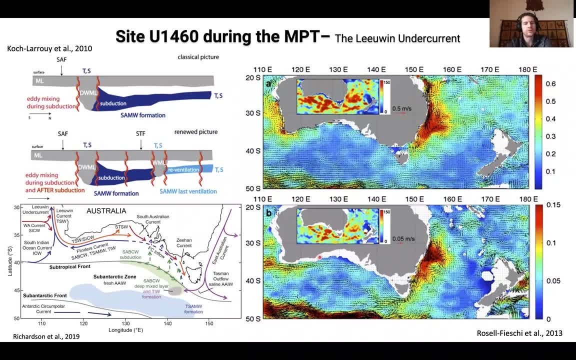 around this area, between the Tasman front and the sub-Antarctic frontal system, around the ACC, which you can see here in this very red and strong current and subducts and then gets transported through the so-called Flinders current along the Great Bight of Australia. 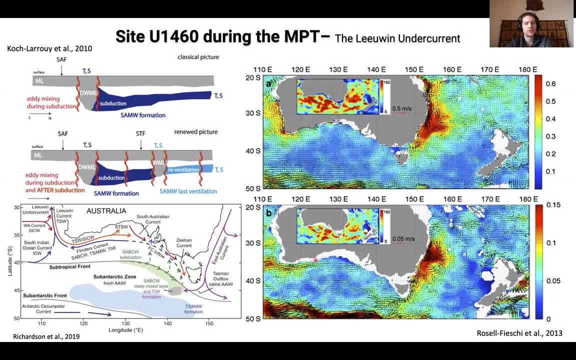 which then flows into the open Indian Ocean But also branches northward towards the so-called Lubin undercurrent, And so there's a direct relation to the amount of sub-Antarctic moat waters that form compared to what we see in the bottom water conditions around U-1460.. 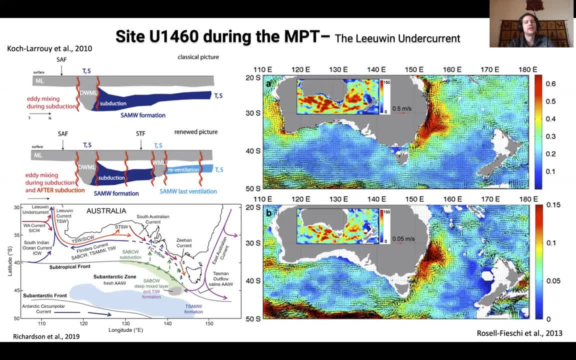 And so our hope is that we can actually improve our understanding of how the equate equate to what? transport of, pardon, of of such sub-Antarctic moat waters and, sorry, in extent also the Antarctic intermediate waters, this form in the Pacific sectors might have changed. 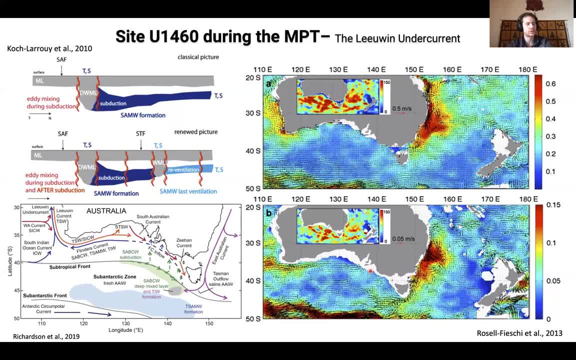 during the NPT. So there we have actually an understanding of our intermediate water circulation that we can then also build upon in our further understanding of what was going on, to this first dramatic sea level ocean during the middle Pleistocene transition and to maybe 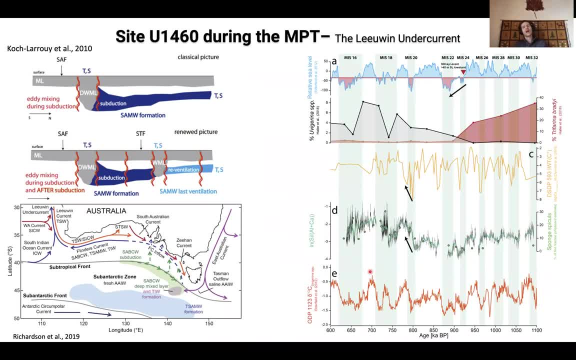 also begin to understand A bit further how this switch from a dominant 41 kilo year, obliquely dominated glacial interglacial cyclicity to the very long 100,000 quasi-periodic cycles of the late Pleistocene occurred. 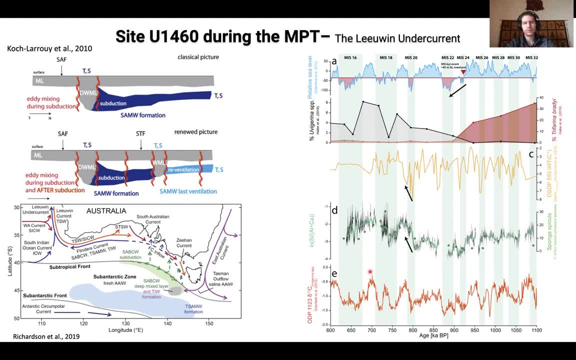 And again, this is ongoing research in progress, and this is also something that my current PhD student is working on, And we're very keen on seeing further data about these things. Good, And this more or less concludes my talk at the moment. 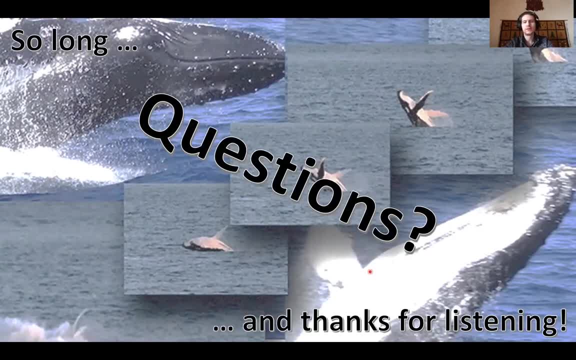 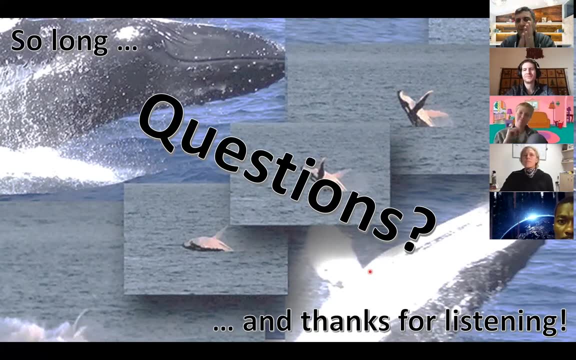 And I would like to thank you all for your attention, And if there are any kind of questions, I am, of course, happy to answer them. Thank you very much for listening. Thank you very much, Gerald, It was really enlightening, And thank you very much. 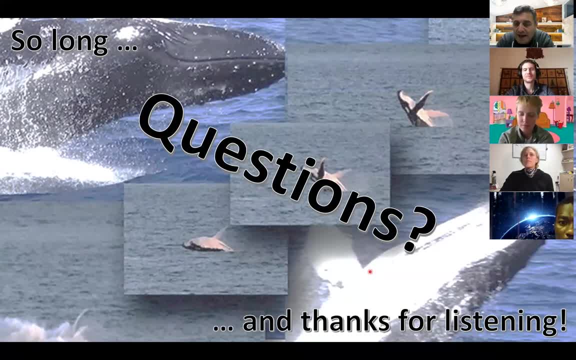 Very informative with a lot of information on the IODP. Thank you, Okay, So I'll open the podium for questions, Since I don't see all the faces. just if you have a question, just go in and interrupt. I think it's the easier. 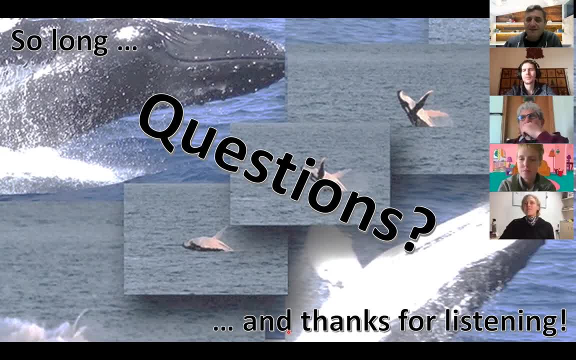 I will ask a question. I will ask a question. I would like to ask a question. Go ahead, Yes. First of all, thank you for the talk. It was a very interesting talk, full of data and interesting data. You've drawn the impacts as if they are completely controlled by the oceanic currents. 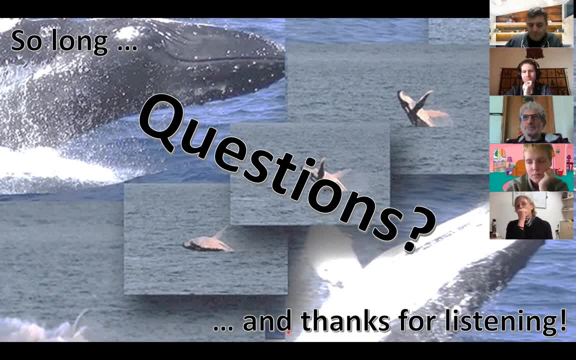 And you are looking on the other end. you're looking along the margin. most of what you've worked with worked along the margin. Is there a modification that is imposed by the margin itself on this? Do you see the modification imposed by the margin on? 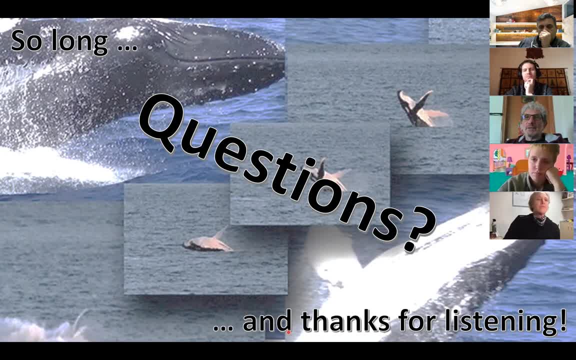 the environment that you're actually examining. Yes, very much so. So our main goal was to basically unpuzzle what was directly related to margin changes for sea level change, and then also what was then additionally going on for ocean or graphic changes. I mean to ask: do you see contribution that? 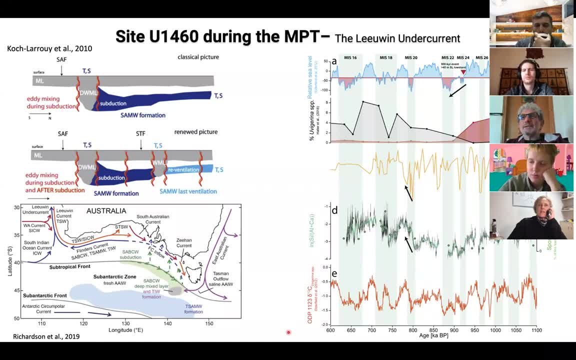 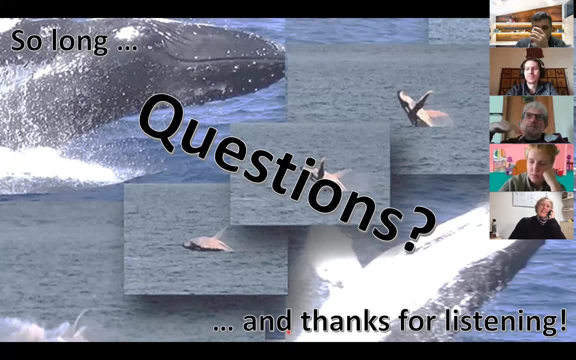 contribute to the productivity, for example, that come from the margin itself, that are associated with the presence of the margin. I mean, does it change the environment, not just the sea level rise? Is there an interaction here, Because you're looking at the deep shallow waster transition? 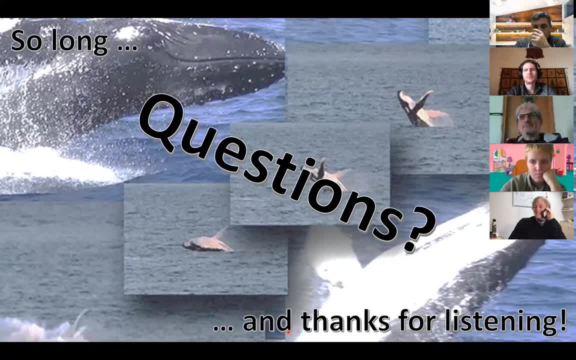 and you should be pumping stuff out of the margin. So you mean just the interaction with the shelf break directly or With the margin? it's not just the shelf, it's the slope also. but yes, With the break area. Does it contribute to your productivity record? do you see a balancing In our understanding? definitely. 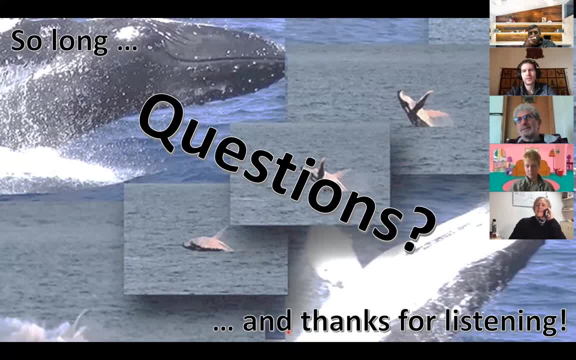 In our understanding, definitely So. do you think it will contribute to your productivity record? do you see a balancing? Yes in our understanding, definitely So. when there is increased Ekman transport, you will get, of course, more nutrients from the margin coming up. 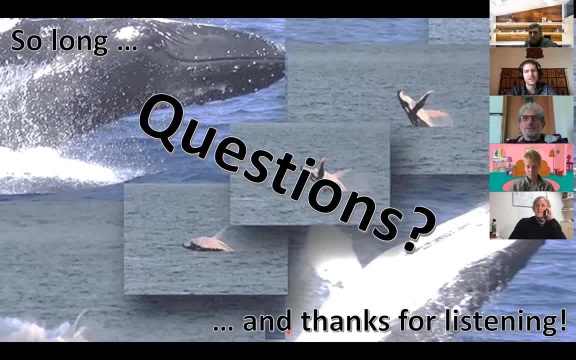 Or do you mean the direct continental contribution, Because this is-. Oh yeah, okay, the Ekman is okay, but do you feel that it mitigates or controls in any way the climatic changes, or is it negligible with respect to the climatic changes?